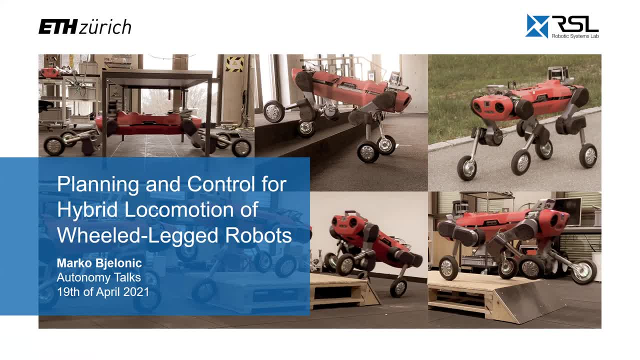 invited some great speakers here, and I'm proud to be part of it, So it's a pleasure also for me to present my work of the last four years, And in the next 40 minutes I'm talking about wheeled-legged robots and their hybrid locomotion skills. But let me first present to you why they will become more. 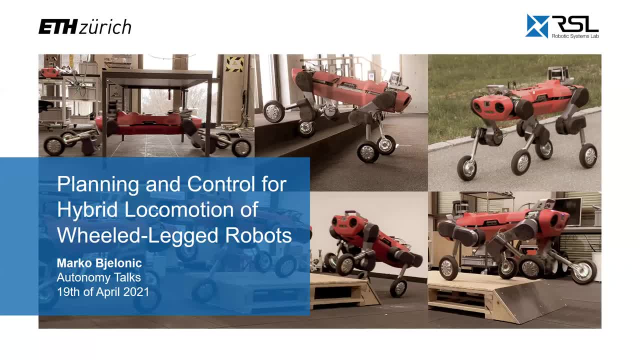 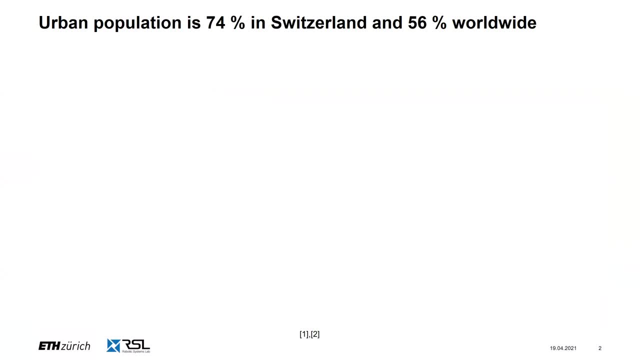 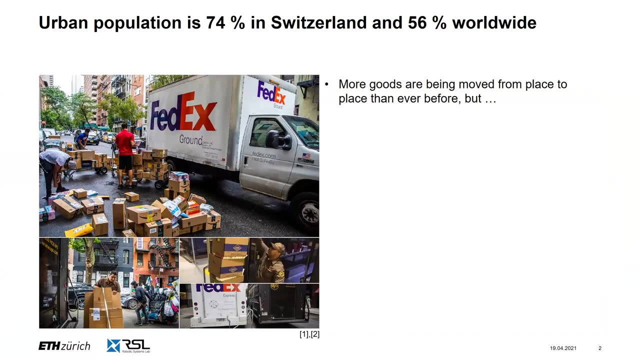 and, more important, Most people live nowadays in urban environments. We can easily foresee that this share will increase even more in the future, requiring smart solutions to make life in cities more livable. In particular, the last mile challenge requires novel ideas that can assist our society with this growing demand. Our fuel-powered 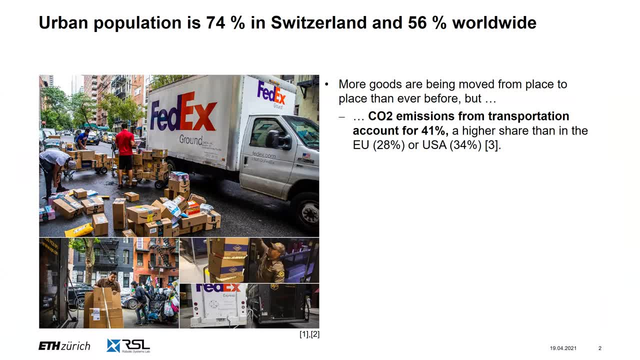 vehicles account for 41% of all CO2 emissions, a higher share than in any other Western countries. Even electrifying this fleet of vehicles cannot solve the problem of increasing traffic congestion and the growing demand for faster delivery. A study by the World Economic Forum forecasts a significant rise in delivery vehicles and therefore emissions in 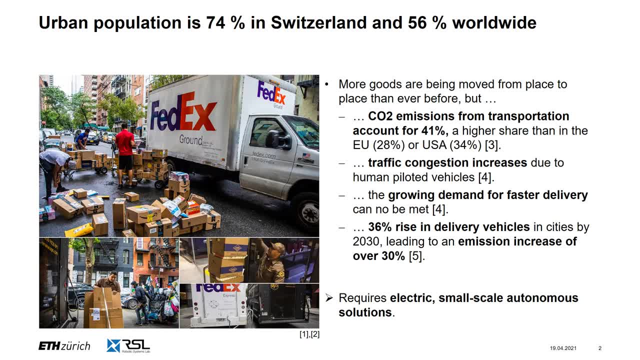 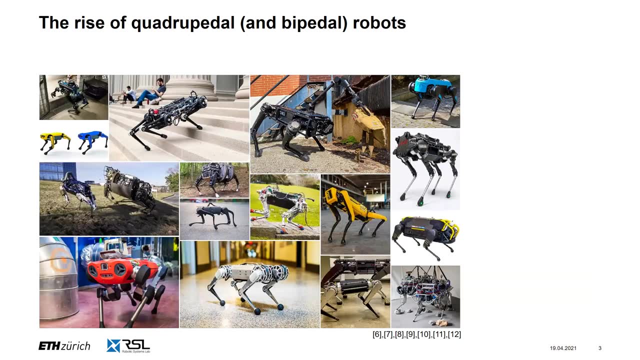 cities by 2030.. For the last mile delivery problem, we believe the shift from human-piloted and fuel-powered vehicles to electric, small-scale autonomous machines would be a global solution. We have seen a rise of quadrupedal robots with similar morphology in the last few years by many 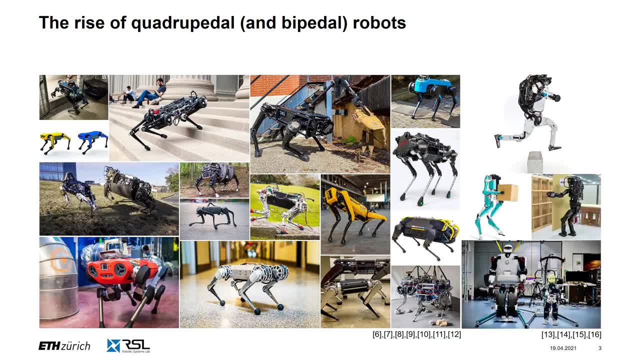 different companies and labs. There are some humanoid robots that can add diversity in terms of the amount of bags. We have seen a rise of quadrupedal robots with similar morphology in the last few years by many different companies and labs. There are some humanoid robots that can add diversity in terms of the amount of bags. 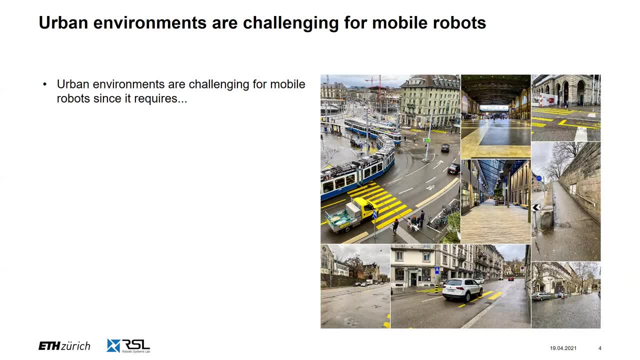 If we look more closely at the last mile delivery problem, a robotic platform operating in cities requires three unique properties. A large part of urban environments consists of flat and open terrains that require speed and efficiency, which cannot be achieved with these traditional legged systems. At the same time, we see a rise of novel six-wheel delivery robots from Starship. 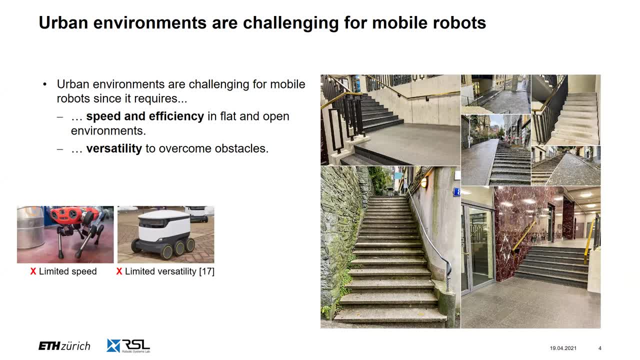 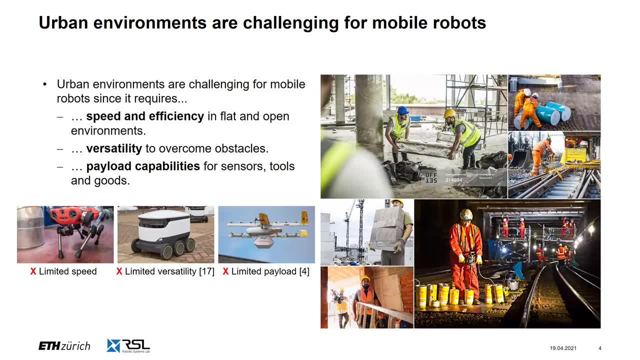 Amazon and FedEx. Urban environments, however, comprise obstacles that their wheel platforms cannot overcome. As an alternative solution, Alphabet's company Wing deploys autonomous lightweight delivery drones to reduce delivery triumphs and greenhouse gas emissions. Wing's payload, however, is only 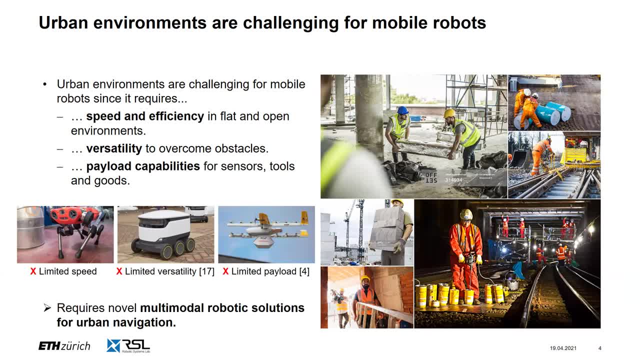 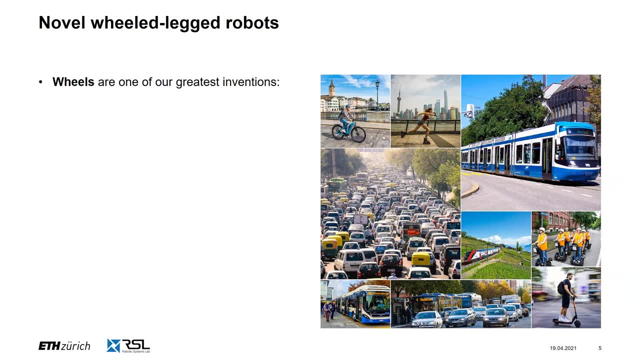 limited to 1.4 kilogram. To achieve speed, versatility and payload capabilities, we need a multi-model robotic solution that allows for individual material transport everywhere. The wheel is one of humankind's greatest inventions that nature could not mimic. Together with humans' unique mobility, the wheel has enabled us to improve the way we live by making 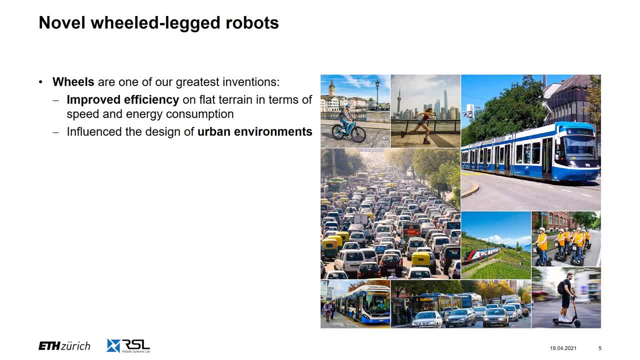 our means of transport more efficient and fast. To this end, we have changed our environments drastically in the last centuries, from terrestrial terrains to relatively flat and open terrains. In these environments, we managed to outperform nature by adding wheeled transportation systems. 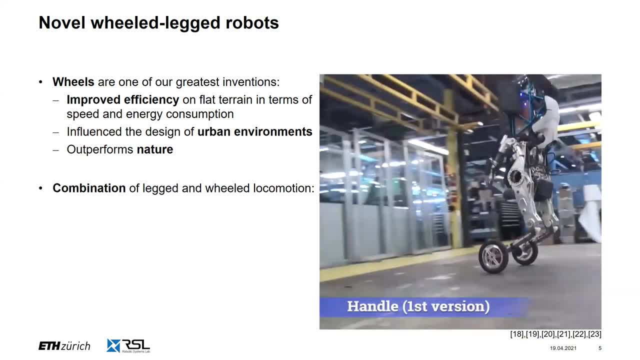 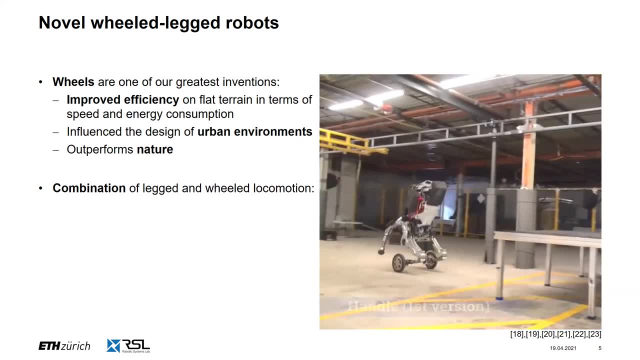 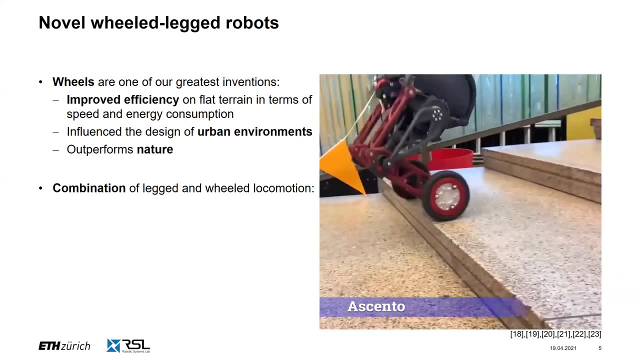 into our daily commute. This inspired the development of these wheeled legged robots, achieving the best of both worlds. The first version of Handle showed impressive motions and the latest version targets logistic applications. Throughout the time of this dissertation, there has been an active 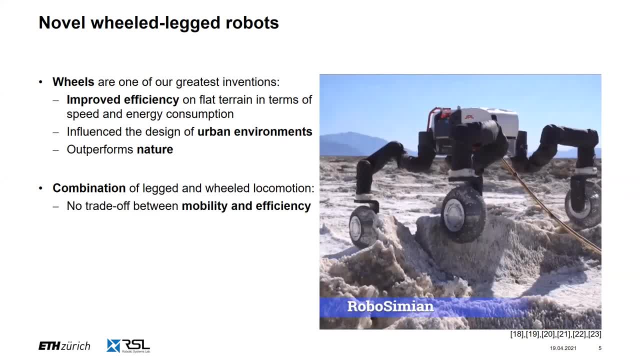 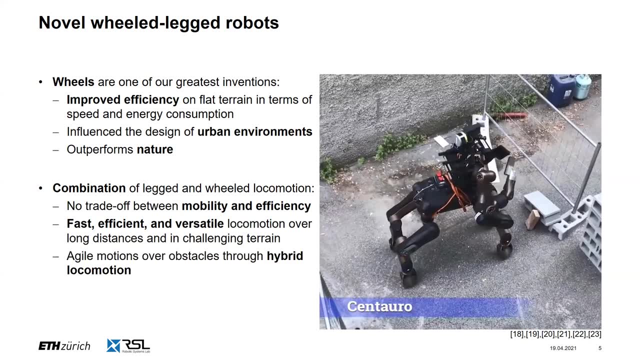 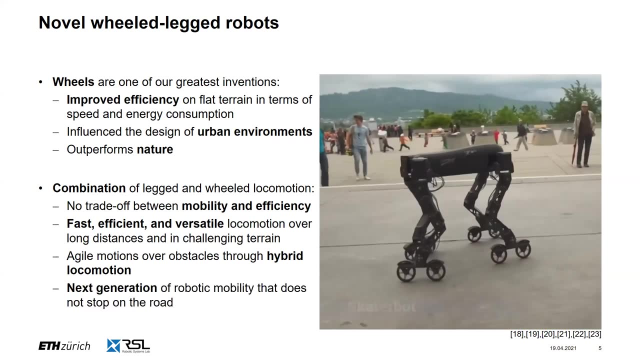 progress in this field. These robots do not have a trade-off between mobility and efficiency, which results in fast, efficient and versatile locomotion. Hybrid motions, where the robot walks and drives at the same time, achieves even agier motions over obstacles. We foresee that this 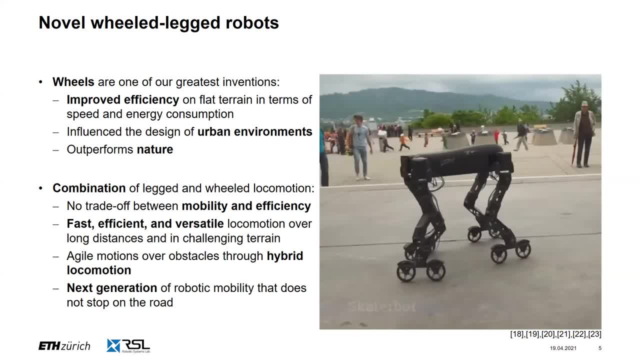 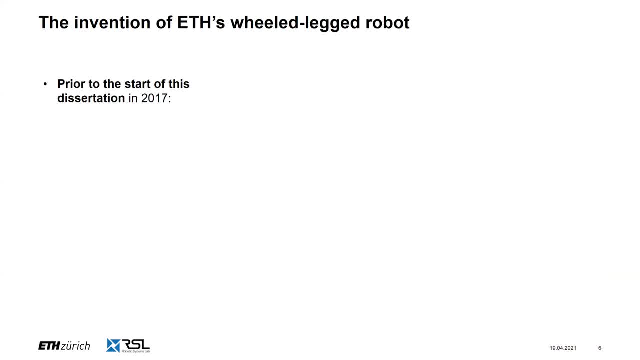 will be the next generation of robots. The road is a new generation of robotic mobility that does not stop on the road. The caveat, however, is that it adds additional complexity through the wheels. I will like to bring this work a little bit into perspective by highlighting the state of the heart. 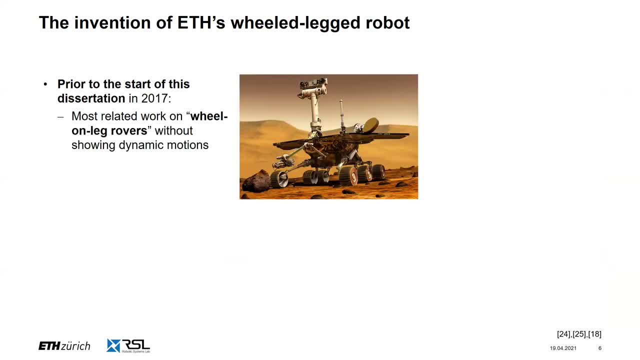 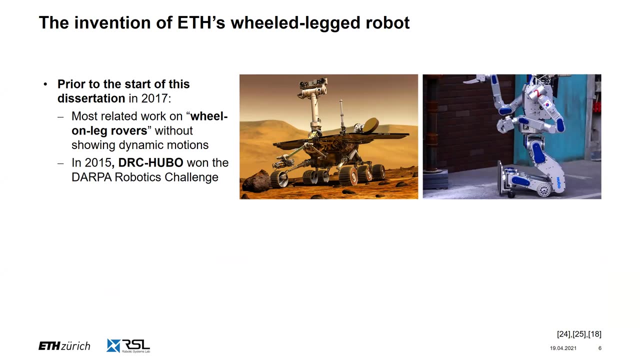 in 2017 when we started working on this project. In the related work, there have been no projects addressing agile wheeled legged locomotion, and research has generally targeted wheel on leg at a suspension system. in 2015, south korea's drc hubo robot won the darpa robotics challenge. 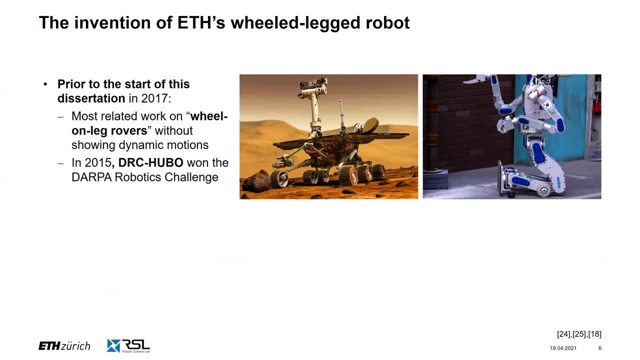 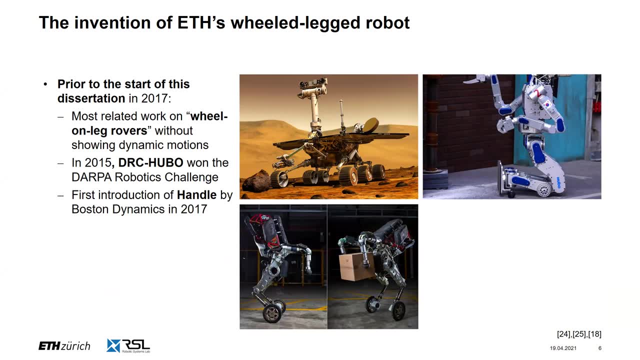 because it was fast and adaptable by switching between driving and walking modes. in 2017, boston dynamics showcased with handle agile motions, where the robot jumps and drives at the same time. meanwhile, we were working on this monster six-wheeled robot with 36 actuators. 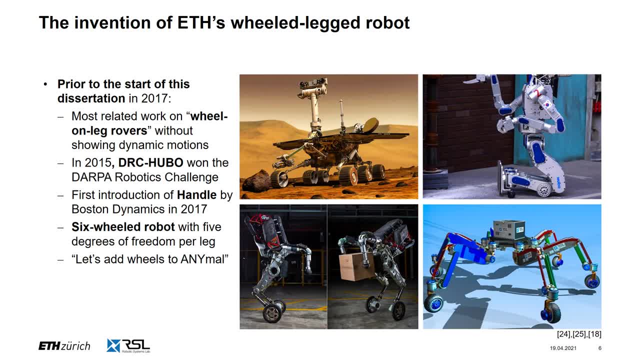 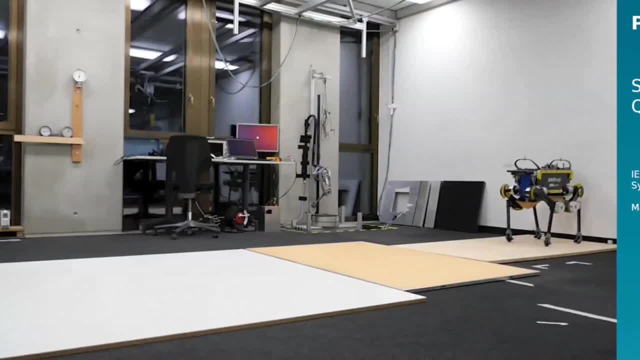 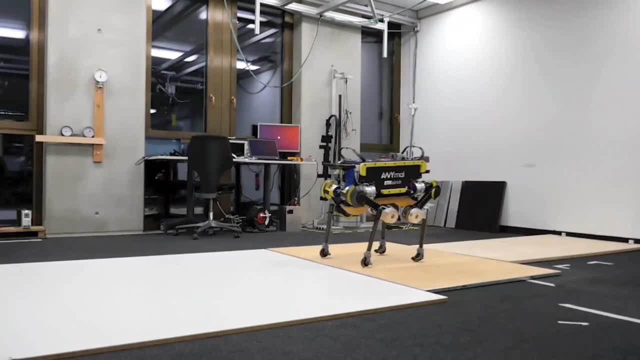 during this development, we changed our direction by adding wheels to our existing quadruped animal. this was probably one of the most critical decisions throughout this study. in 2017, we showcased skating motions with passive wheels, and throughout this presentation, you will experience how much the robot's capabilities improve compared to its very first version. 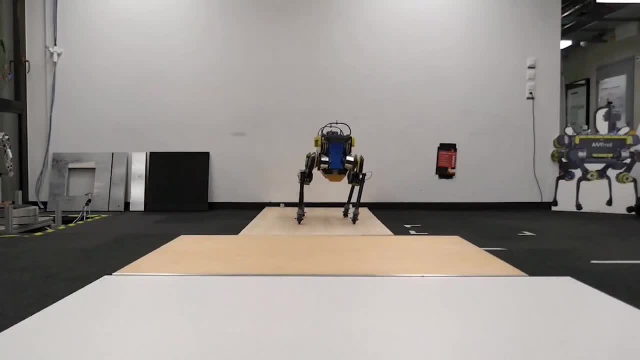 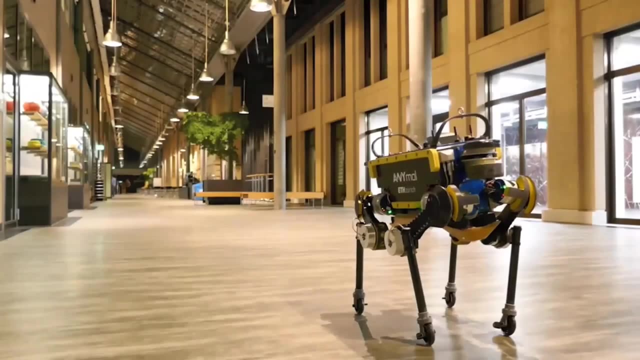 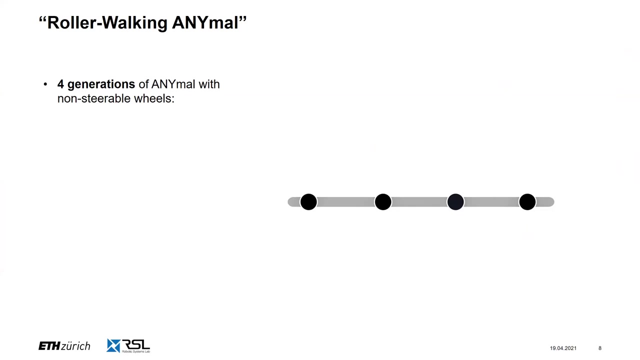 one of the interesting aspects when controlling skating motions is that legs cannot produce any ground reaction forces along the rolling direction and due to the robot's kinematics. we add a clause with which the robot can generate forces to propel itself. our lab released four generations of our of the 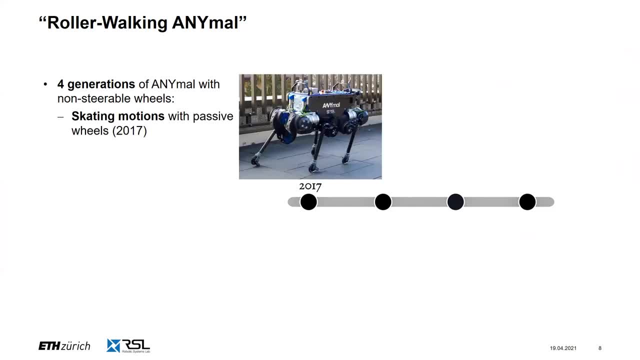 roller walking animal over the last four years, as shown in the previous video. the first version showed for the first time skating motions with passive wheels. in 2018, we switched to powered wheels with a maximum torque of four newton meters- the key difference between a human 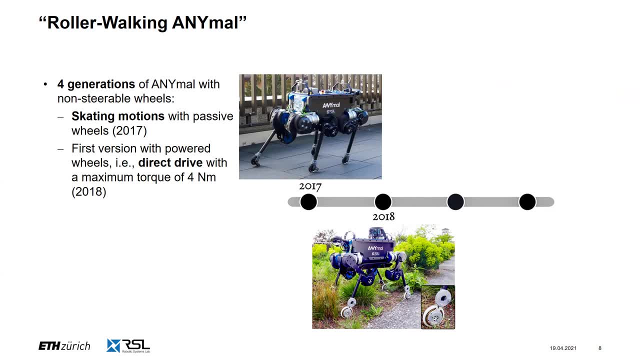 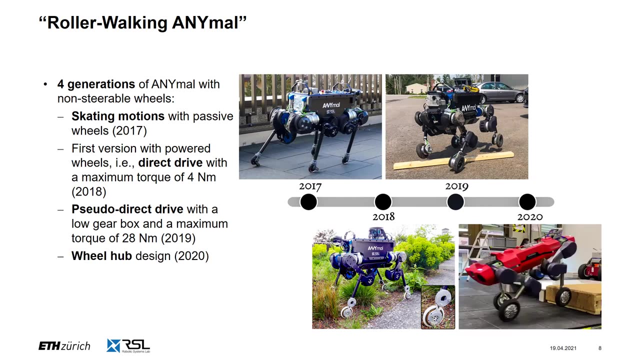 wheel and a robot equipped with activated wheels is that the robot can exert control over its wheels that human cannot match. we quickly noticed that the wheels torque was not enough and we upgraded to a pseudo drive: drive with 28 newton meters in 2019 and the wheel hub design in 2020. 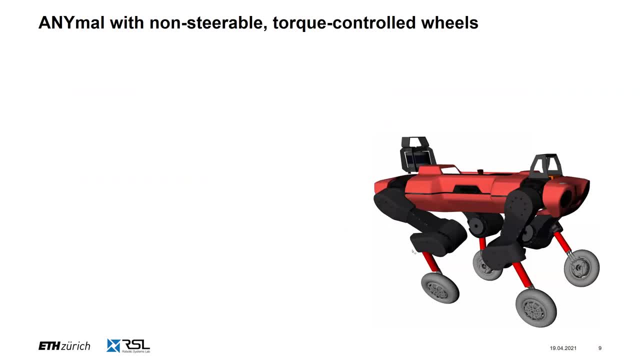 if we look more closely at our final version of activated wheels, then we can identify 16 actuator degrees of freedom, where four of them are part of the non-serial wheels. due to this design, the robot needs to execute hybrid locomotion in order to turn and pure. 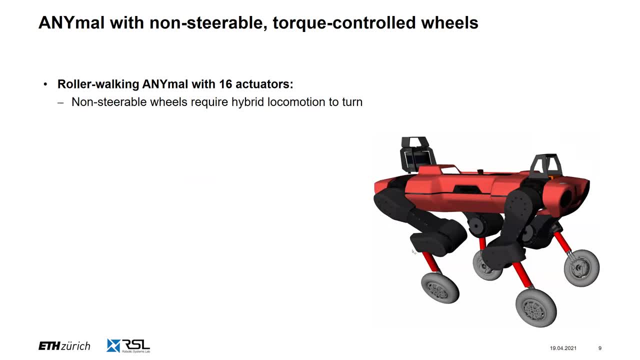 driving motions are only possible along the robot's forward and backward direction. the weed-legged robot also requires a stat, a state estimation of the robot's pose that considers moving ground context. to deal with uncertainties of the terrain and state estimates, we torque control all actuators, but how can we generate the torque commands for all of these actuators? 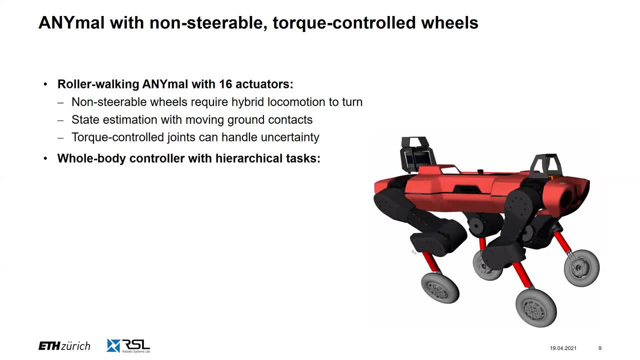 by applying a whole body controller that considers the full rigid body dynamics and tasks such as inequality, constraints that respect the friction cone and torque limits and the rolling constraints. that basically states that acceleration at the contact point equals a centripetal acceleration. we can track contact forces and other whole body trajectories. finally, the feed forward torque is: 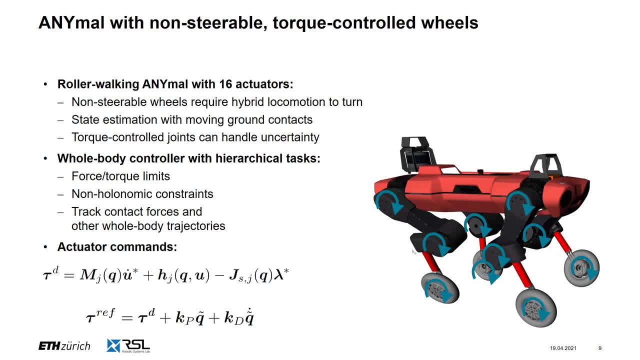 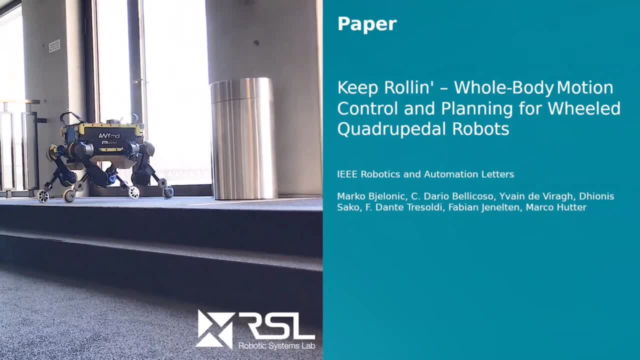 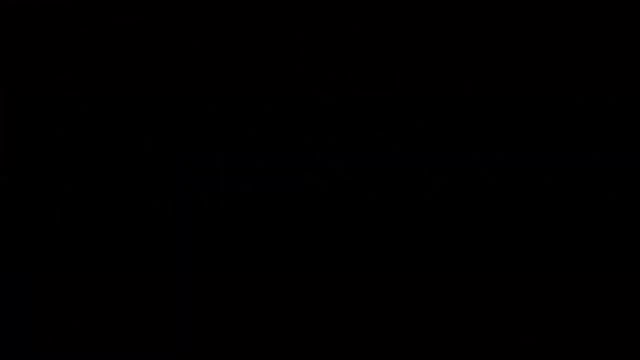 computed with the full rigid body dynamics and with some low gain, position and velocity tracking, we can account for modalities. With this approach, we can adapt to unforeseen conditions, as shown here, where the robot with the vector-treated wheels drives down stairs blindly. The robot has no information about the change in contact size but because of the torque 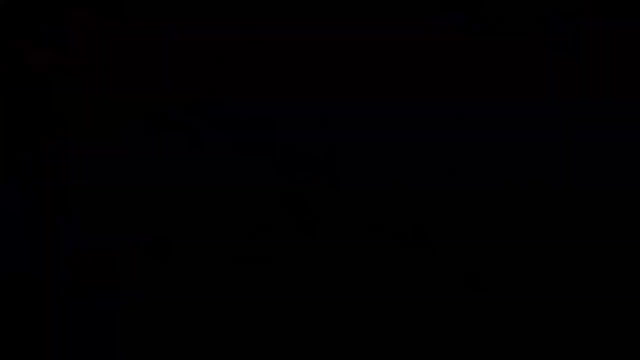 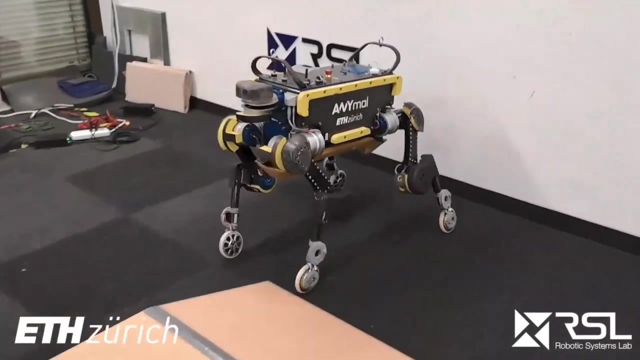 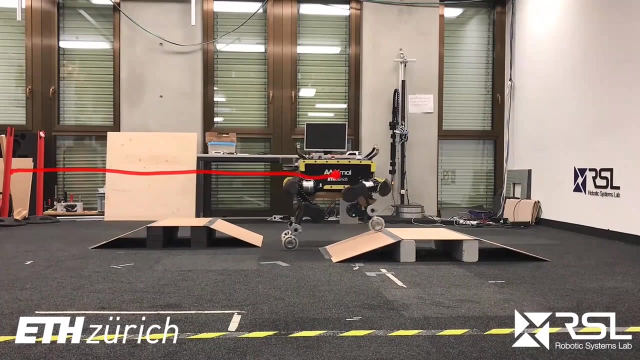 control approach through the whole body controller, we can react to it. The robot can even react to these bumps blindly with 0.7 meters per second, while keeping its torso level and adapting only its legs. With this whole body controller, we can even add arbitrarily other limbs to the robot, as 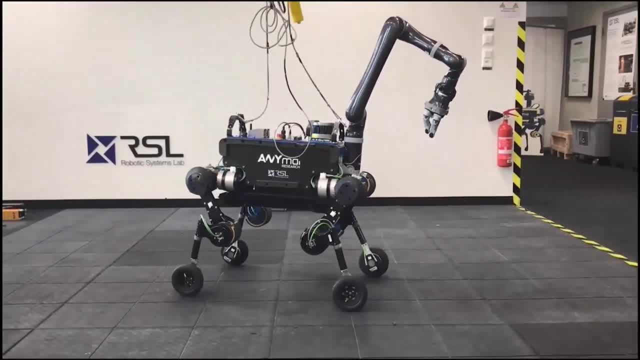 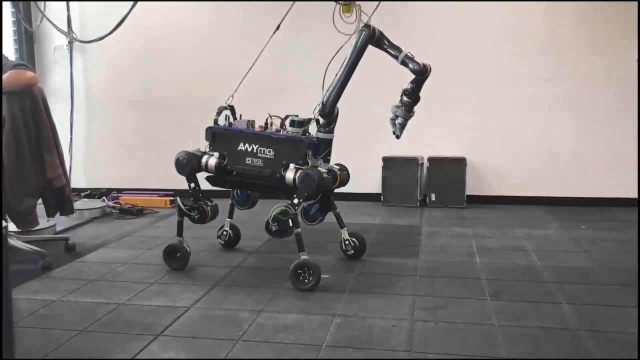 shown here, where we extended the robot with an arm, where the task is to keep the arms and the vector fixed with respect to the world frame or some base frame, as shown here. But if we want to overcome challenging obstacles, as shown here, we need to expertly plan the 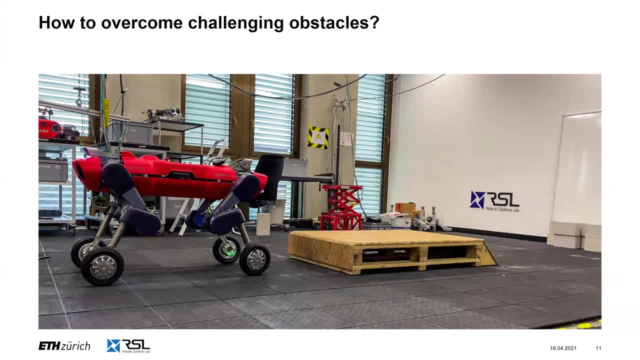 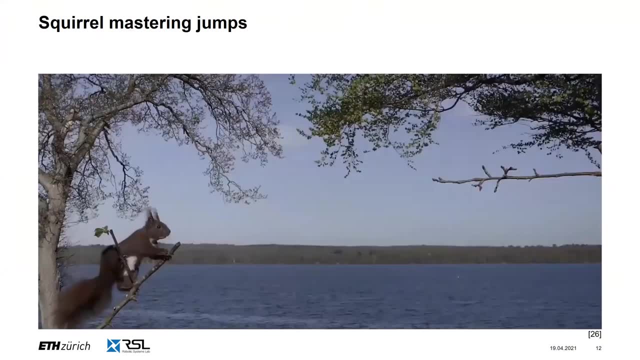 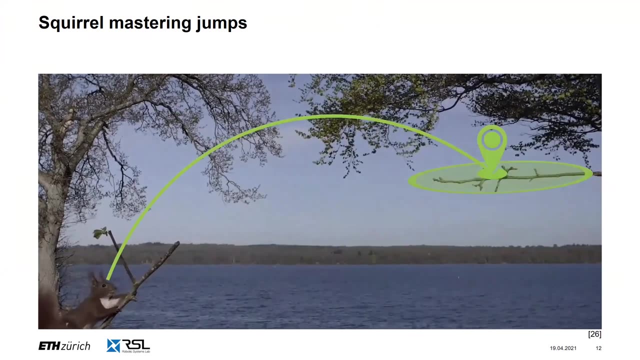 robot's future actions, while considering its multi-modal skills. So how can we achieve this? To answer this question, let's see how a squirrel is mastering jumps. We can see how it investigates the starting and goal branch. With this information, it can pre-compute and predict its future motions before execution. 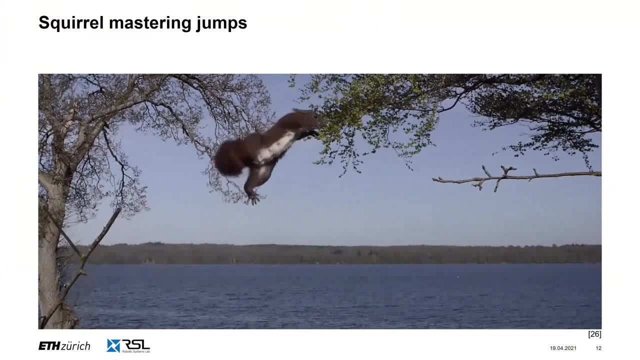 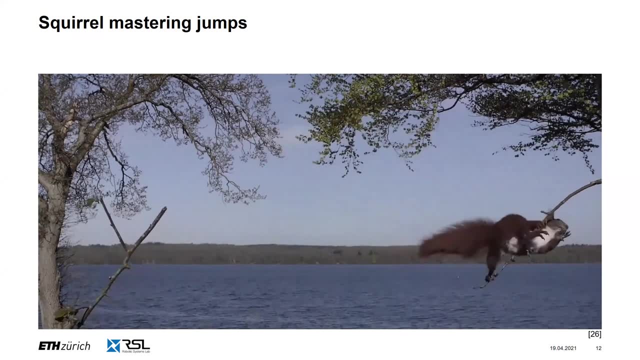 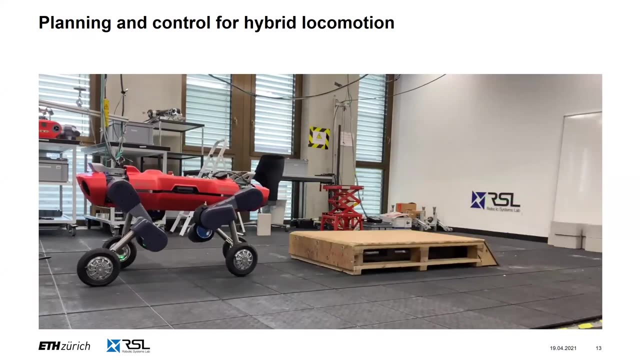 During execution, it can correct its initial movement over a shorter horizon towards the goal And even though the branch, as you will see, now bends quite a bit, the squirrel can react and successfully finish the motion Inspired by the squirrel's synchronization of fast interactions and look-ahead planning. 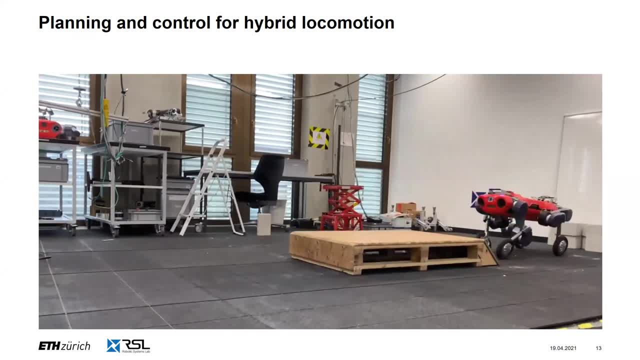 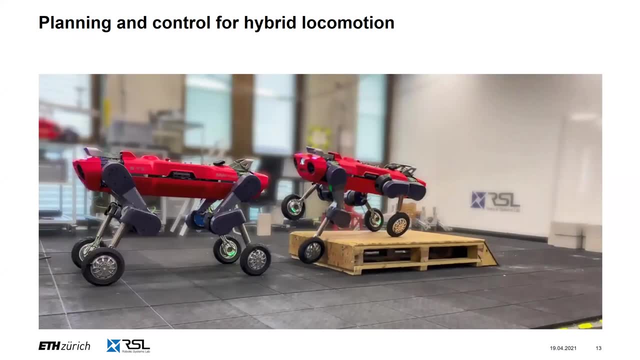 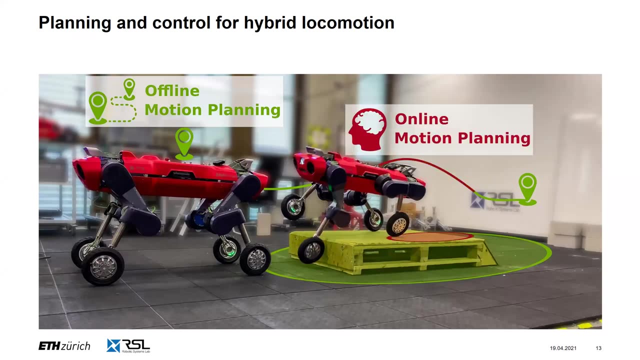 our robot can achieve agile motions over this wooden box. To this end, we developed an optimization-based framework that first transforms high-level tasks offline into complex motions over a longer time horizon And then, during the execution, an online motion planner optimizes along the offline trajectories while considering a shorter 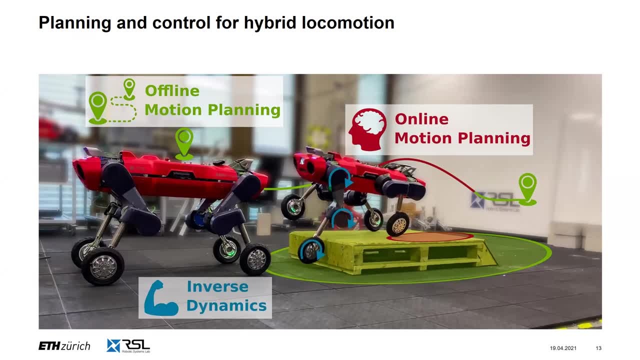 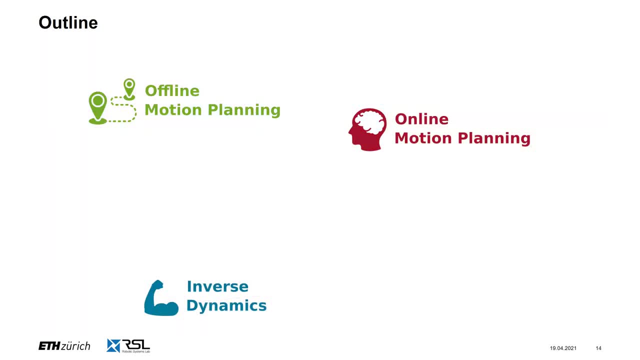 time horizon. Finally, at each control cycle, we compute torque commands through inverse dynamics that are fed to the robot. Let's put these three blocks together and see how they interact. First, the offline motion planner generates an offline trajectory, which is fed into the 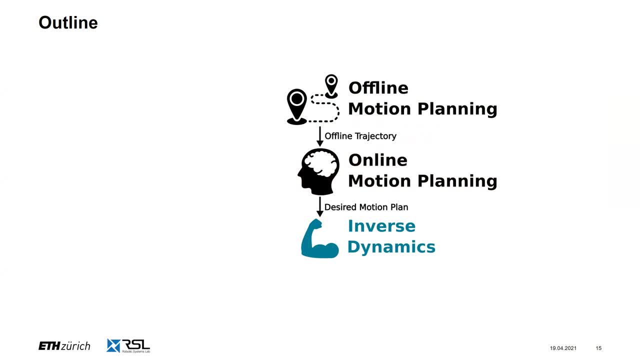 online motion planner that continuously optimizes a trajectory with a shorter horizon that is fed into the inverse dynamics. The last module sends torque commands to the robot And with these three modules we can generate dynamic motions over obstacles, as shown here. The remaining part of this presentation focuses on the motion planning aspect, considering 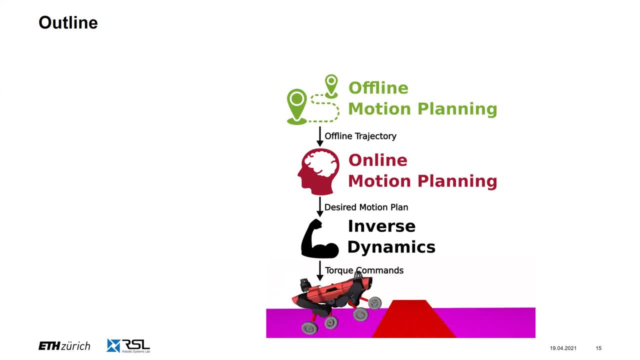 the robot's future trajectory, since it remains an open research program. Let me first discuss the online motion planning stage, here highlighted in red. Here we consider a shorter look-ahead. The robot is designed to plan reactive behavior and explore task simplifications due to the 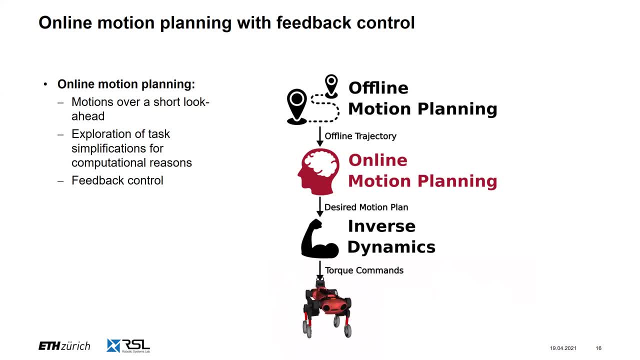 read-time requirements on the robot. The online motion planner robustifies motions to a certain degree by recomputing solutions on-the-fly and adding feedback control. This visualization, for example, shows the robot's future torso and read trajectories over a one-second time horizon. 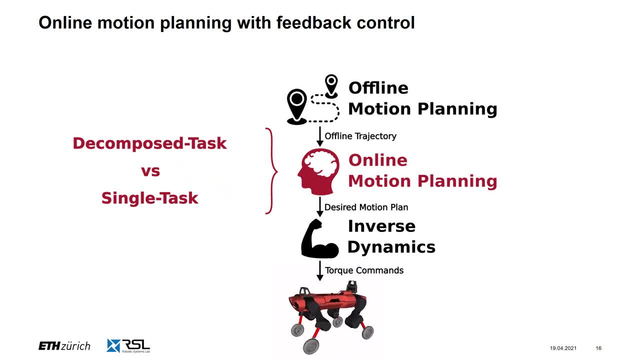 In our work we compare two motion planning concepts: 1. Torso Task and Single Task Planner. The former breaks down the high-dimensional planning problem into lower-dimensional wheel and torso subtasks, which make the individual problem more tractable than a single optimization and can be solved at a faster update rate. 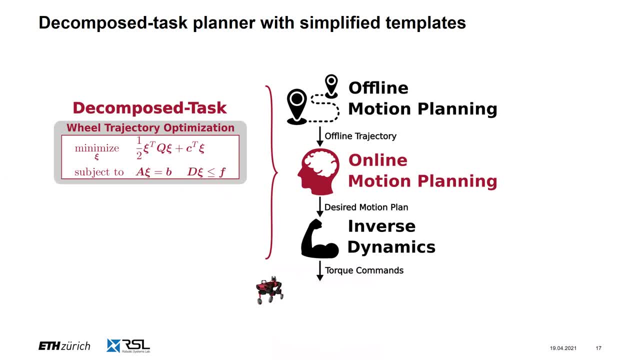 compared to single-task approaches. The wheel trajectories are computed in a QP, where we minimize a quadratic cost function subjected to linear constraints. Meanwhile, the torso optimization becomes a nonlinear optimization. With this approach, the update rates are in the order of hundreds of seconds. 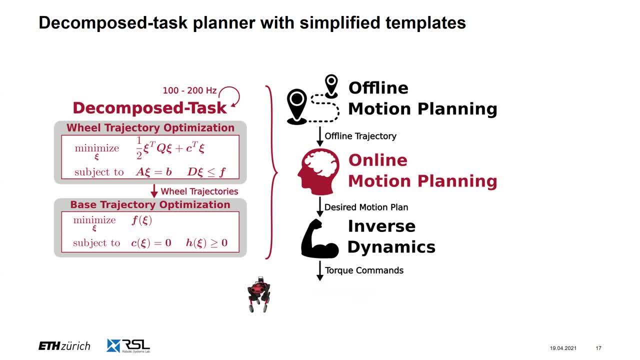 The coordination of each task's solutions, however, is one of the main challenges, and heuristics are needed to align the wheel and torso motions, which prevents us from tracking complex offline trajectories, and therefore to evaluate our decomposed planner. we merely 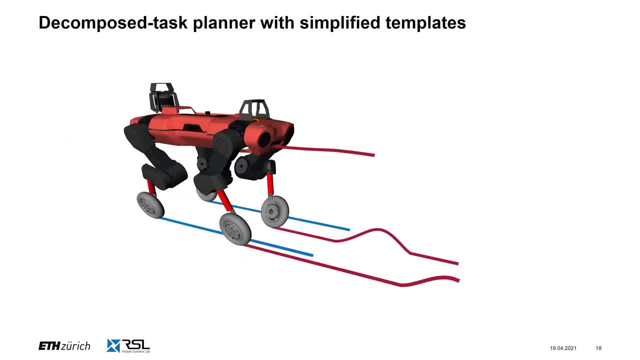 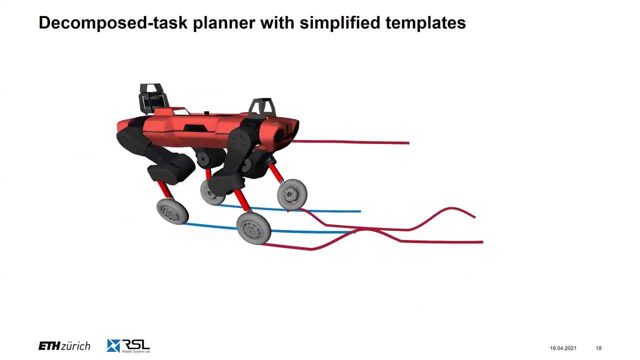 follow velocity commands from an operator. So let's have a closer look where these heuristics come from. 1. Torso Task and Single Task Planner. The common method in legged locomotion designs foothold positions based on the inverted pendulum model, where Pleg is the reference foothold. 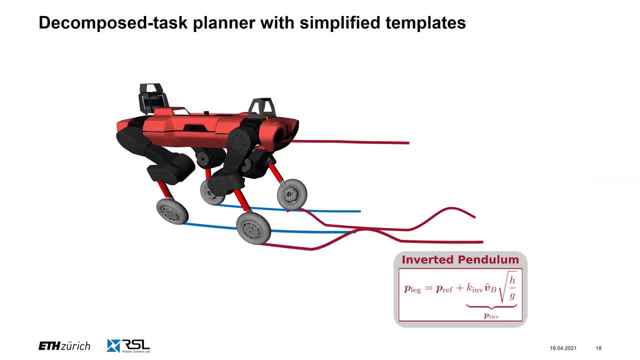 position that is split into feedforward reference signal, Pref, and a feedback term that is based on the velocity error of the torso Vb, together with the feedback gain K, the robot's height h and the gravitational acceleration g. 2. Torso Task and Single Task Planner. Given the hybrid wheel trajectories we sample. 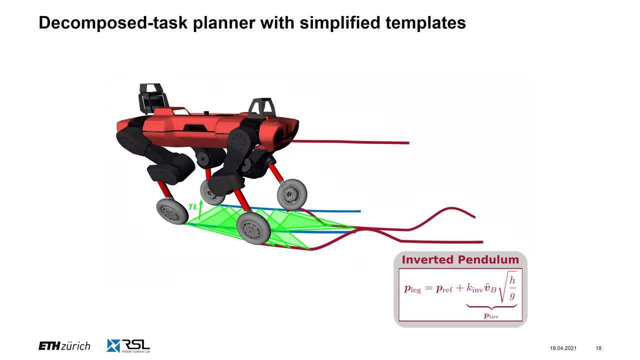 the future support polygons of the wheels which are here, the green triangles. Here the center of mass motion is approximated by the gravitational inertia branch F and M which acts as a substitute for the contact forces. With this branch and terrain, normal N, we can compute the zero-moment point constraint. 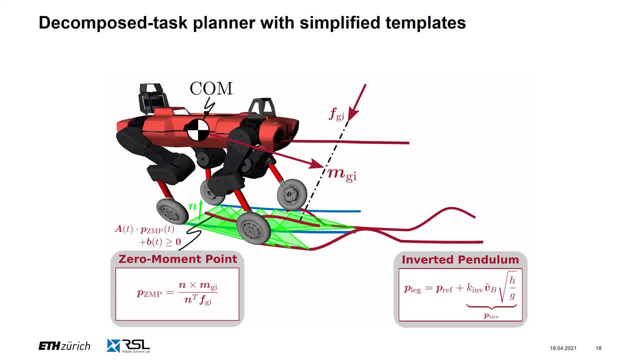 which is considered to lie inside the support polygon. 3. Torso Task and Single Task Planner. To summarize, the wheel trajectories and torso projections are connected through these two motion templates And, as we will see in a bit, the wheel trajectories can diverge from the torso trajectory and 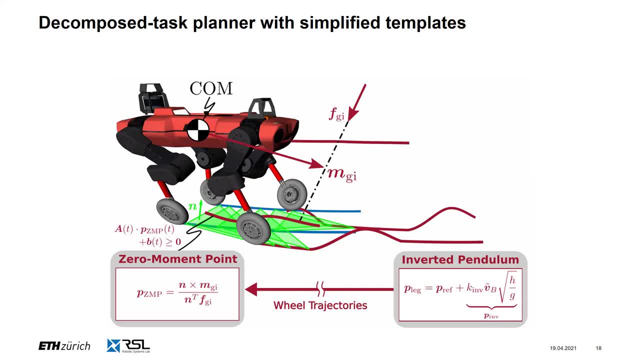 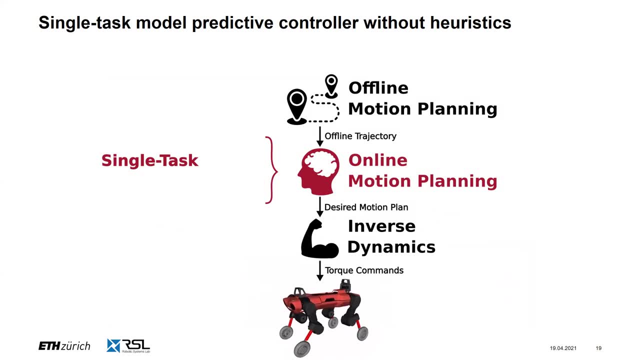 it is quite difficult to handcraft an inverted pendulum template for a wheel-legged robot that captures hybrid locomotion. In contrast, a single-task approach treats the continuous decision problem as a whole without breaking down the problem. Here the challenge is to solve the problem in a reasonable time so that online execution 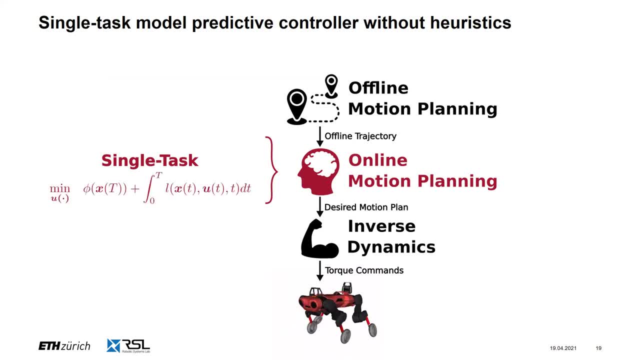 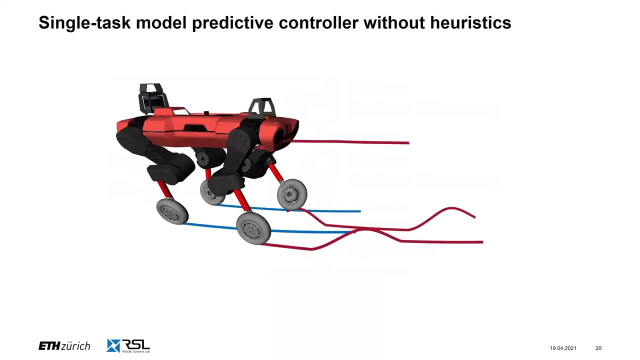 on the real robot becomes feasible. To this end, we introduce an MPC for wheel-legged robots. Since the single-task approach optimizes over a larger number of variables, the update rate becomes 20-50 Hertz. We will now present the model predictive controller that solves the coordination problem of the 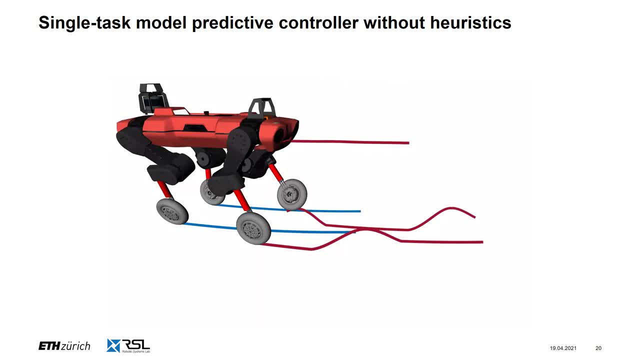 decomposed task approach by treating the hybrid locomotion problem as a whole without any heuristics. Here we minimize the cost function that is involved. Here we minimize the cost function that is involved. Here we minimize the cost function that is involved. 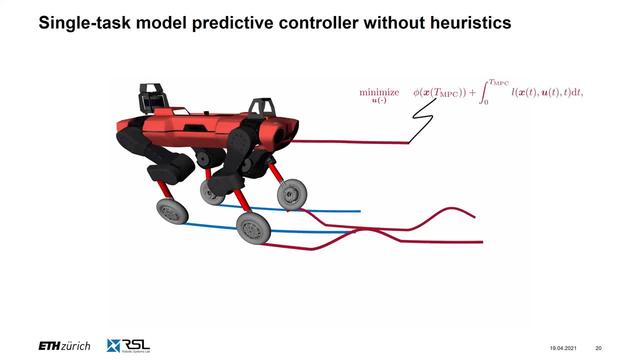 For example, theêt functional view of a frame is defined internally in terms of how much material is included, bearing running cost L, which is a function of the state vector x, and control input vector u. The state vector x is the 6-dimensional pose and twist of the torso and also includes 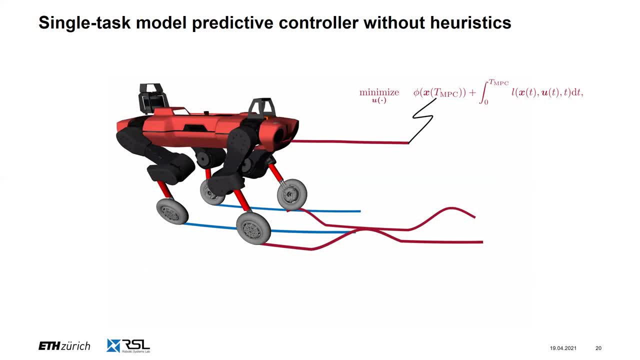 the joint positions. The control inputs are the contact forces and joint velocities. Since we are considering the robot's full kinematics, we can define the system's dynamics as a kinodynamic model, which is important, as we'll see in the next slide. 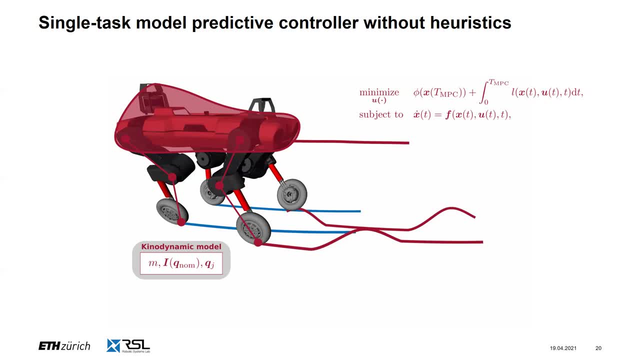 It defines a single rigid body dynamics with mass M, inertia I, along with the kinematics for each leg qj. At each iteration of the MPC we update the MPC's initial state with the robot's measured state. We can add equality constraints where we can say that swinging legs have zero contact forces. 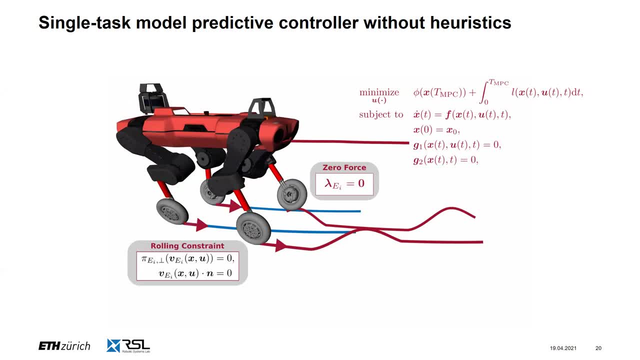 and grounded legs can only generate velocities along the wheel's rolling direction. We will visualize this constraint in more detail in the next slide. The traversal of challenging terrain requires additional inequality constraints that respect safe terrain regions. To this end, we add half-space constraints a and b of the end-effector position Pe. 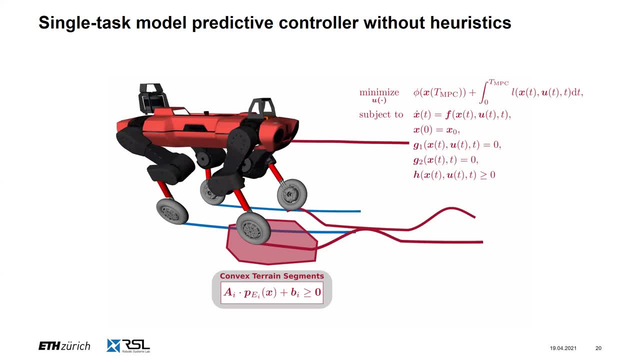 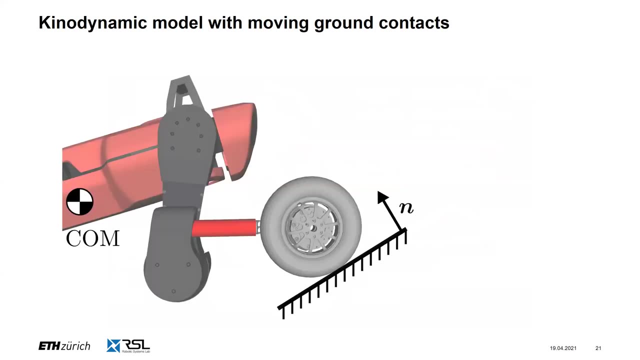 that ensure the grounded end-effectors to stay inside the safe terrain. We can add friction cone, inequality, constraints of the contact forces, lambda and collision avoidance with the environment of the end-effectors m and b and torso. So let's have a closer look at the rolling constraint As shown in this sketch. 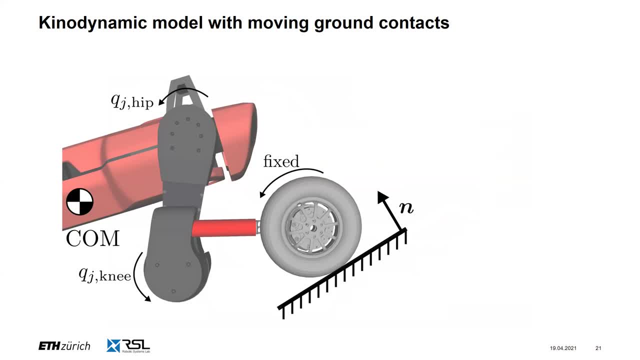 we model the robot's wheel as a moving point, contact, with a fixed joint position, while optimizing the legs, remaining kinematics and considering the size of the wheels. By expressing the wheel, the rolling constraint, in a way that this red velocity is set to zero and also this blue velocity sideways to the rolling direction, we can let the optimization 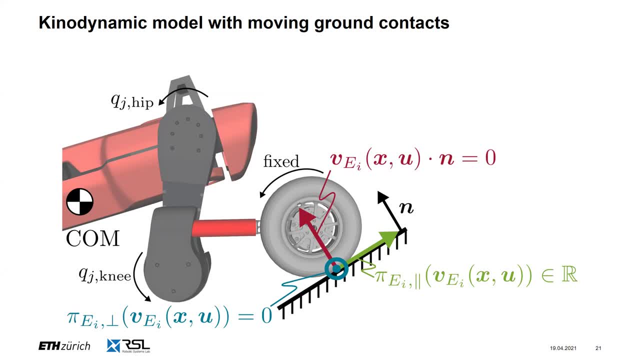 explore motions along the green velocity vector without any heuristics. All of these three projections onto the three different directions and the end effectors- contact position, Re- can be easily computed in the MPC through forward kinematics and does not require any simplification of the robot's rolling direction, which is actually needed in a decomposed approach. 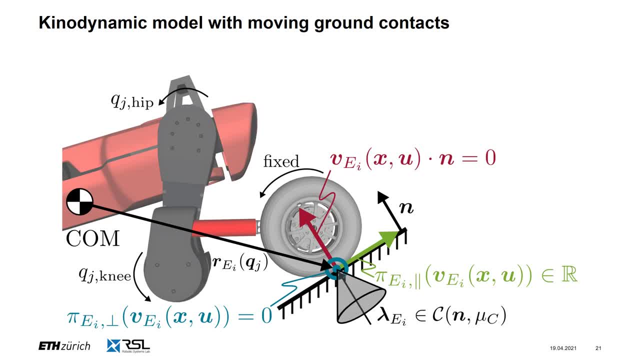 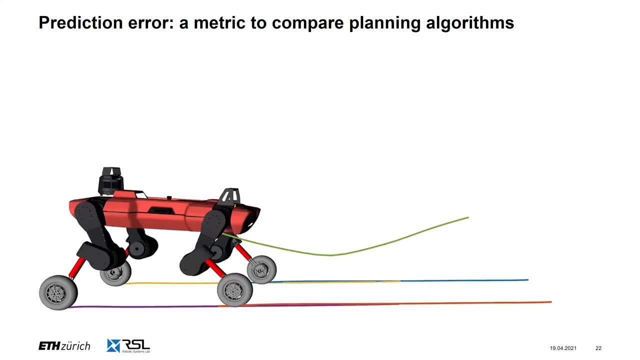 In the same way as we deal with traditional legged robots. we can add the friction cone constraint and any other constraint to this moving point Point contact. So quantitatively comparing receding horizon planners based on the real robot's performance is a non-trivial task. Our work provides a quantity that describes how well a receding 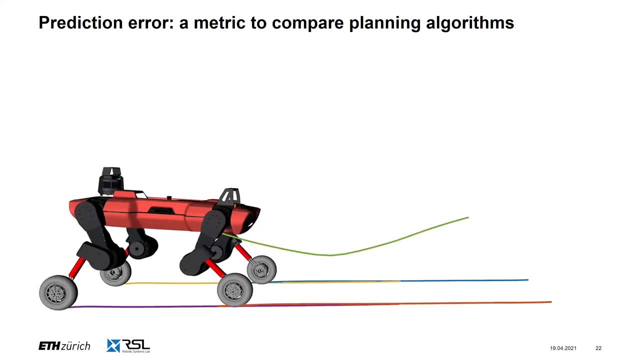 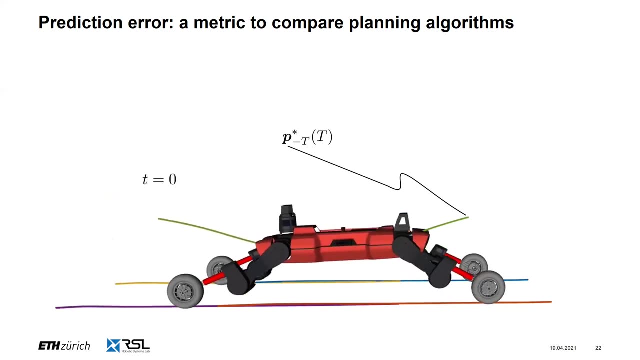 horizon planner can predict the robot's future state. So let's say we have the future trajectory of the robot and to evaluate how good the trajectory's underlying model approximates the real robot, we compute the final state of the trajectory at the beginning And execute the planner over one horizon. capital T. 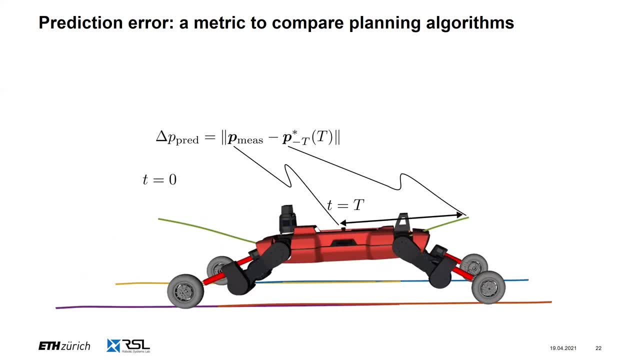 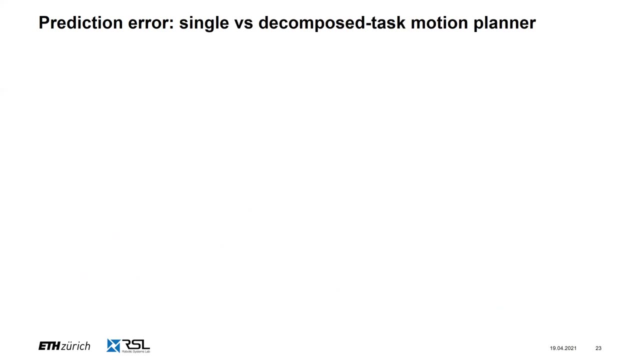 Now we can measure what the robot's actual state is And by comparing the measured state and the predicted state, we can compute this prediction error, which is only valid if the commanded reference velocities were constant over this executed duration. We use this metric to compare. 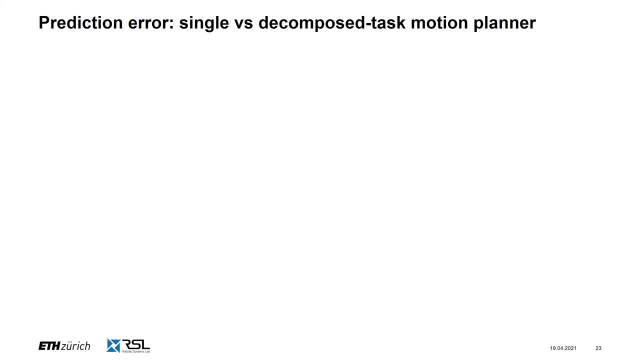 the prediction accuracy of the decomposed and single-task motion planner on the real robot. Moreover, we can use this metric to compare the prediction accuracy of the decomposed and single-task motion planner on the real robot. Moreover, we plot the prediction accuracy on the z-axis over linear and angular velocity commands. 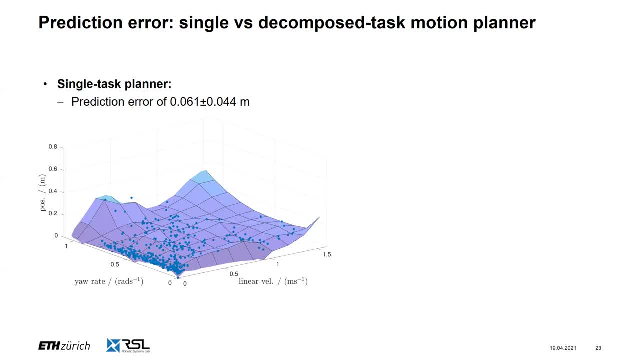 The goal for any planner is to achieve a low value and, as we can see here, the single-task approach achieves a relatively constant prediction error over this range of velocities. A comparison with the decomposed approach on the right shows that the single-task approach on the 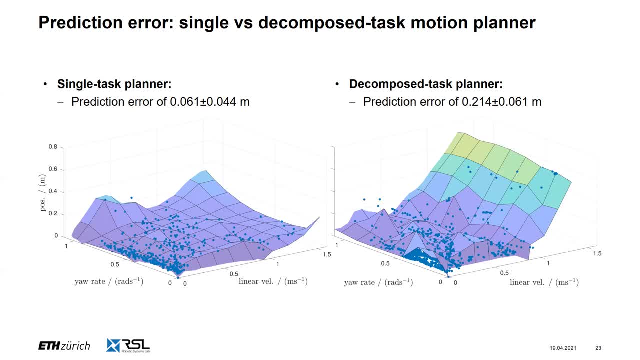 left can predict the robot's future trajectory more accurately. Especially at higher commanded velocities, the prediction error is more accurate. The prediction error of the decomposed approach increases drastically, which is also the reason why this approach fails at higher speeds. Our single-task approach solves the problem and improves the prediction accuracy by up to 71%, making fast locomotion feasible. 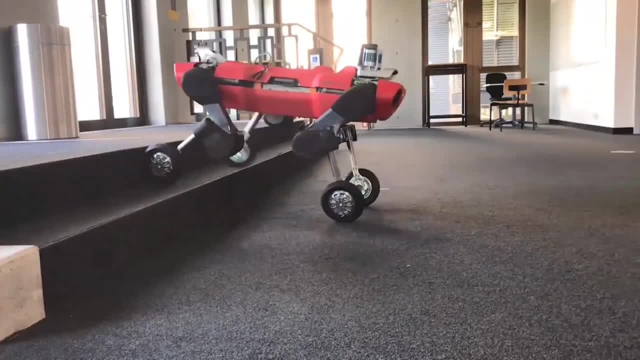 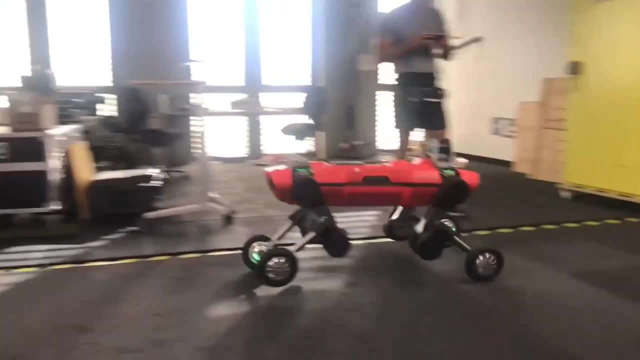 With this single-task MPC we can accurately capture the robots, dynamics and rolling constraints, enabling us to execute novel hybrid motions. Here we show some fast acceleration where the single task can be done with the original effect. find some interesting solutions to quickly change its erection. 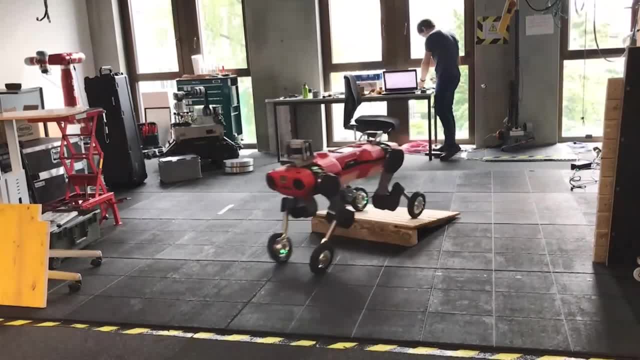 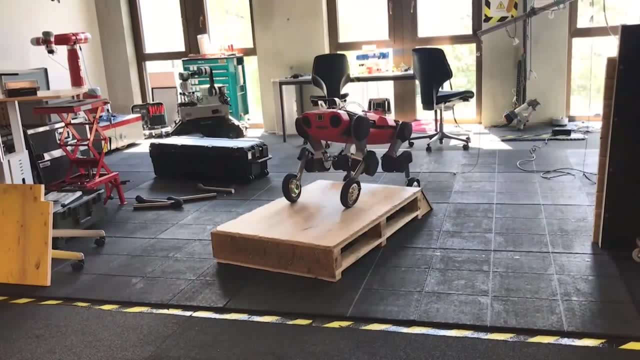 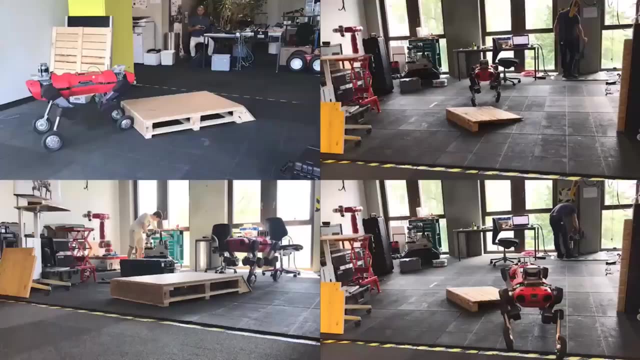 Such motions are not feasible with the decomposed approach In this video. the robot is still blind and has no prior knowledge of the obstacles. Nevertheless, the robot can smoothly adapt to stairs and steps. Moreover, we verified the approach over a high variety of obstacles and also gates. 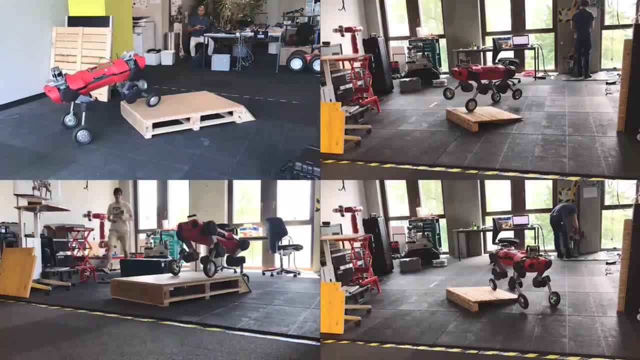 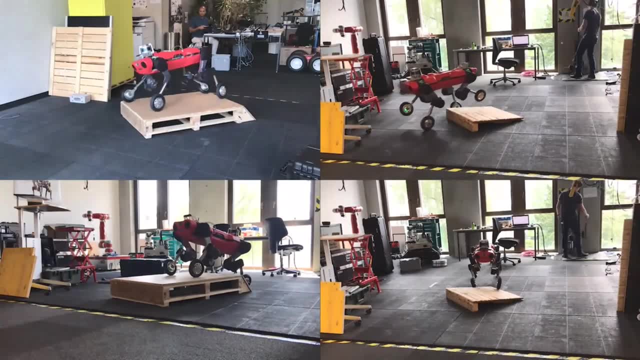 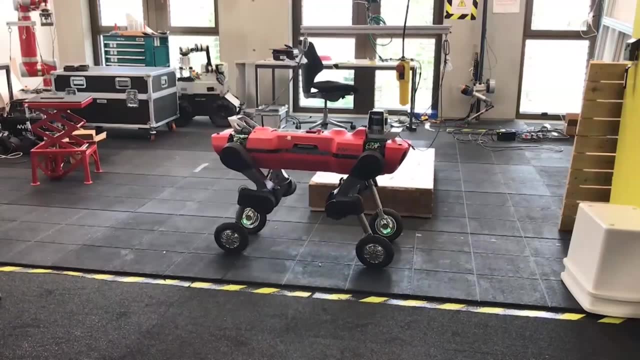 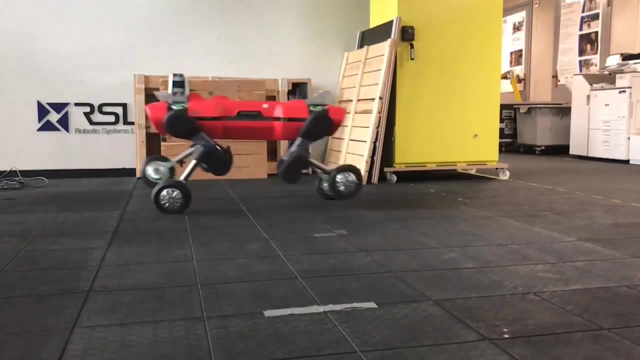 where the robot executes hybrid or pure driving motions, as shown here. In addition, we can also perform some dynamic jump with the front legs, where the algorithm automatically commands the grounded legs to support the dynamic motion. One big improvement of the single-task approach is that we can execute all motions and gates. 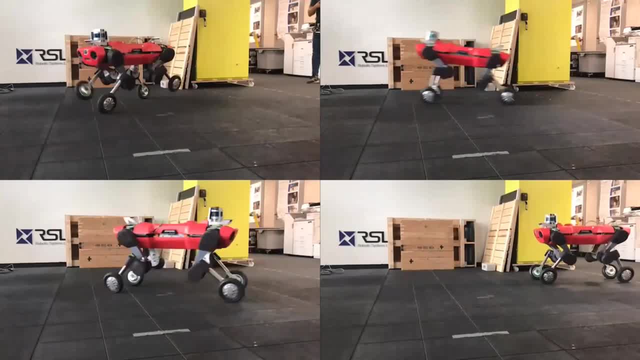 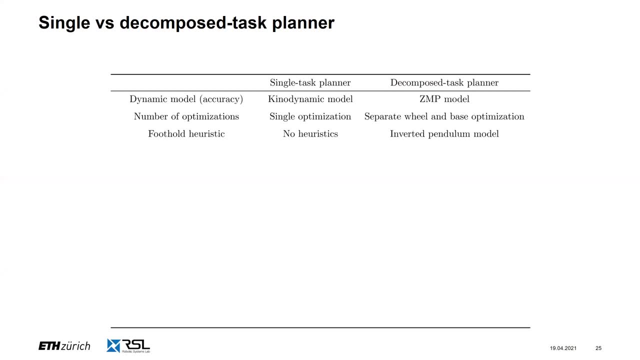 with a single set of parameters, as shown here. So let me briefly summarize the takeaways from this study. Here we can see side by side the used dynamic model, the number of optimizations and the foothold heuristic. Obviously, the update rate drops when optimizing all states in a single optimization. 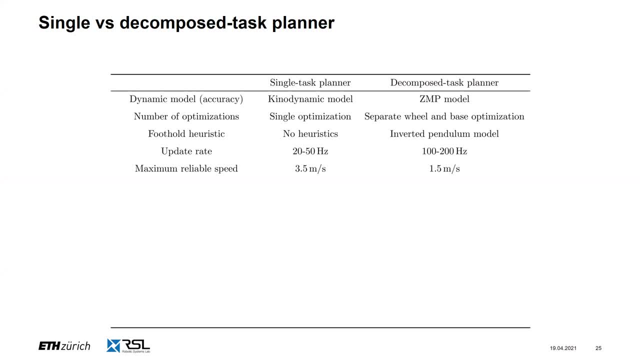 which is acceptable considering the robot's reactive behavior performance shown in the video before, and we managed to have a higher maximum speed compared to the decomposed task approach. We achieved this by optimizing over more states in a single task and also by including the contact forces. 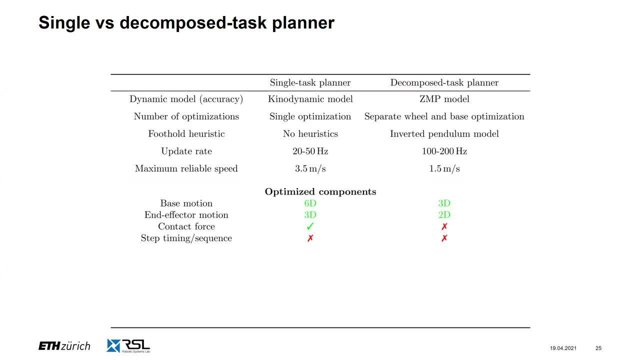 Both optimization problems do not optimize over the step timings or sequences In general, increasing the algorithm's complexity improves the difficulty of shown tasks. When we look at the achieved tasks, the last task is quite important for weed-legged robots and can only be achieved with the single-task approach. 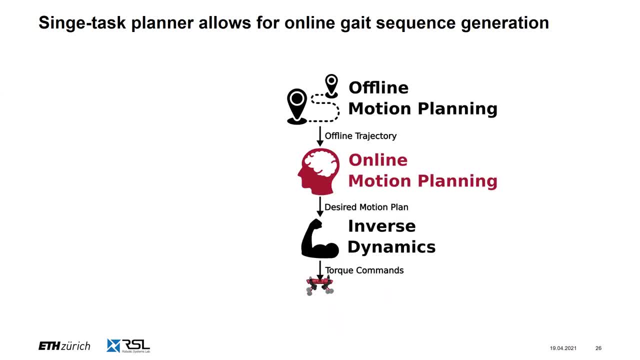 The visualized motion below represents a fixed hybrid trotting gate, which is not optimal from an energetic point of view, because by only lifting the legs when needed and maximizing the time spent driving, we can lower the cost of transport. To this end, we showcase an approach that, based on the velocity commands. 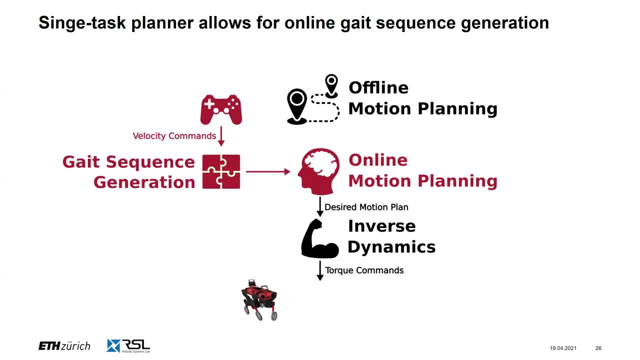 adapts the online planner's gate sequence. This can only be achieved in combination with the single-task MPC, since it uses a single set of parameters for all motions. We tested an online gate sequence generation in Wangen an der Ader, where the robot locomotes under the Ader. 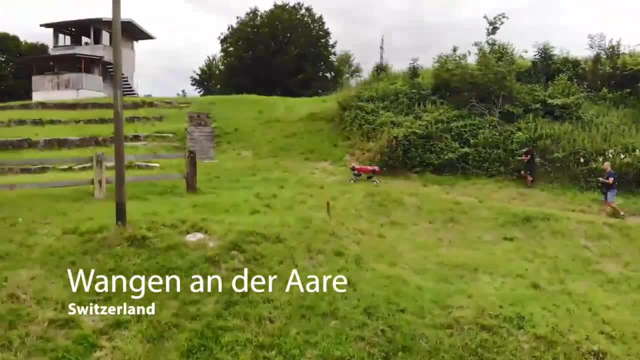 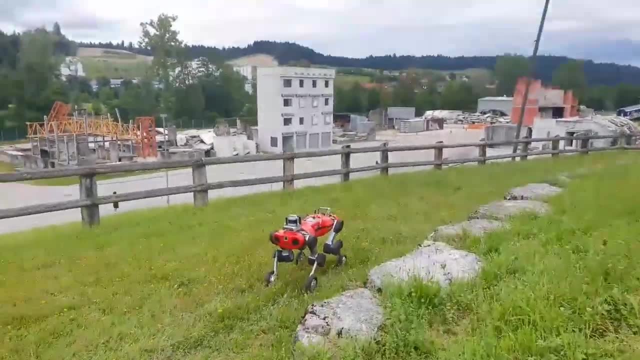 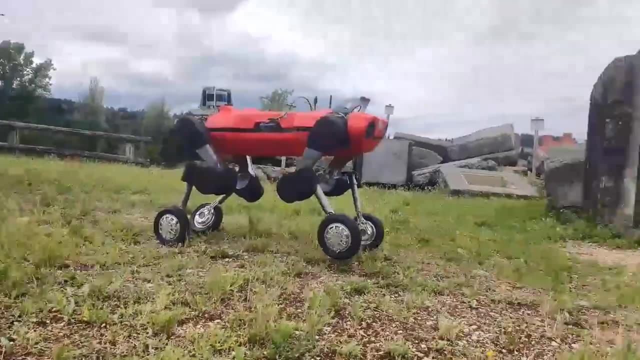 the robot locomotes up a grassy hill and continues to move on paved roads. Being able to switch between pure driving and stepping can increase the locomotion's efficiency dramatically. This concept therefore quantifies kinematic lag utilities for online gate sequence generations of the MPC's timings. 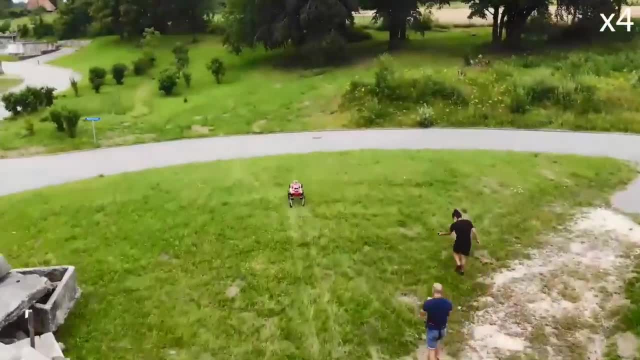 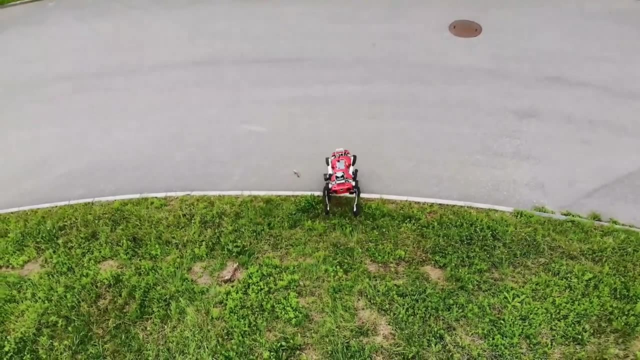 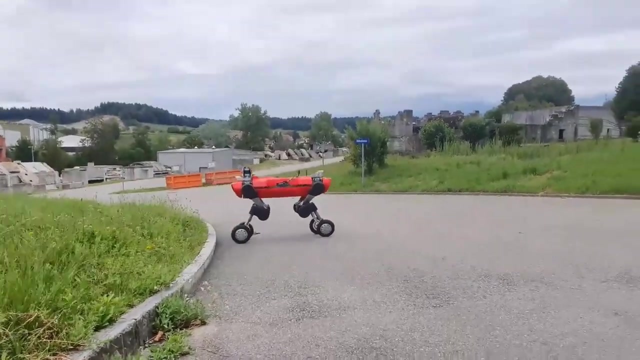 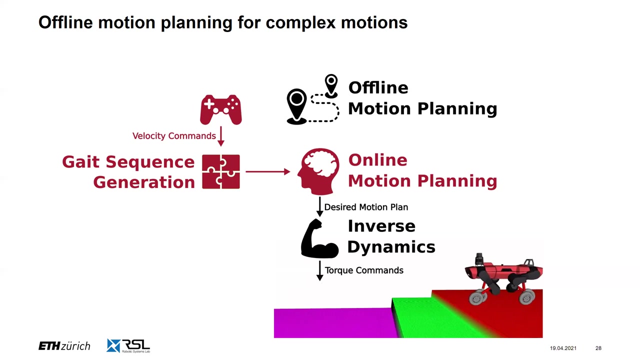 without the need for predefined contact timings and lift-off sequences. This automatic gate discovery enables our weed-legged robot with non-sealable wheels to coordinate operatic behavior and reduce the cost of transport drastically. The execution of more challenging obstacles, as shown here below. 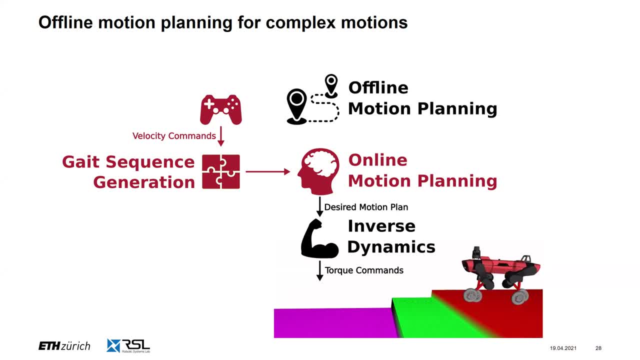 requires the integration of the gate timings into the motion planning. In most cases, such a holistic approach, optimizing over more optimization variables, may not be feasible to run online on the robot. To achieve this, we run these motion planning algorithms offline before execution. Thus motion planning of these two steps requires more complex optimizations. 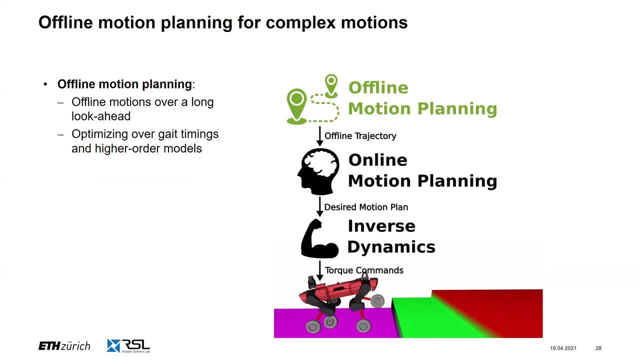 over longer time horizons, Considering more realistic models and variables like step timings. this allows us to generate complex motions at the robot's limits. Such complex optimizations, however, suffer from longer optimization times and require our single-task online planner to robustly execute these offline trajectories. 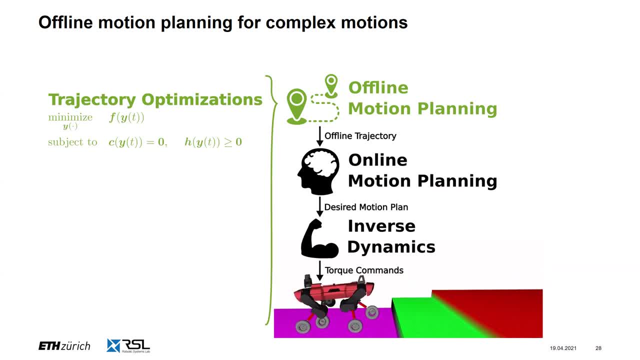 Let's have a closer look into the offline planning stage. First, we use trajectory optimizations that minimize a nonlinear function f that is subjected to nonlinear equality and inequality constraint c and h. These algorithms transform high-level tasks like a goal pose given a height map. 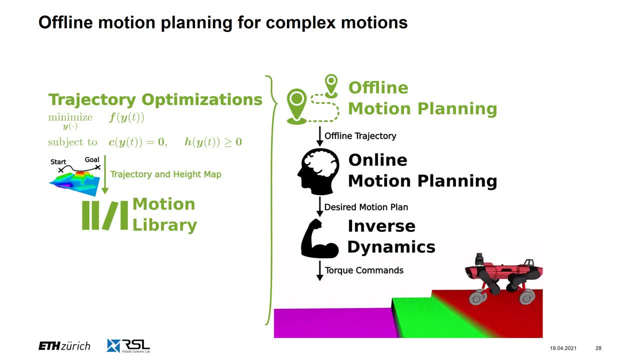 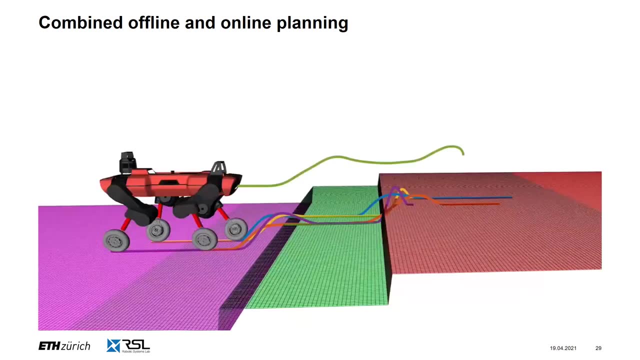 into dynamically feasible motions which are stored in a motion library. An operator can choose individual motions from this library online and each of these motions can be composed together, resulting in even longer maneuvers. In the following, we discussed the interaction between offline and online planning. 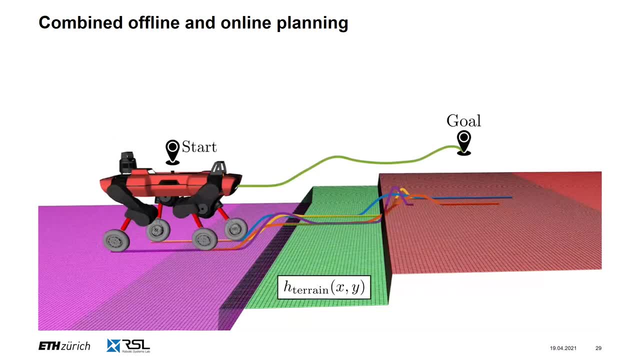 This visualization shows the robot before executing the motion, Given the desired start and goal position, including the terrain's height map. the trajectory optimization generates the offline trajectory. For readability reasons, we split the offline trajectory into the state vector xto, and control input vector uto. 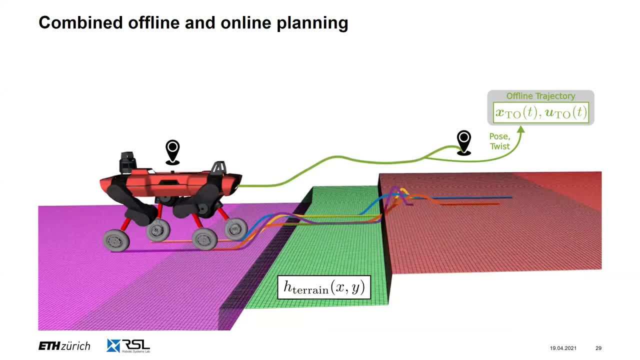 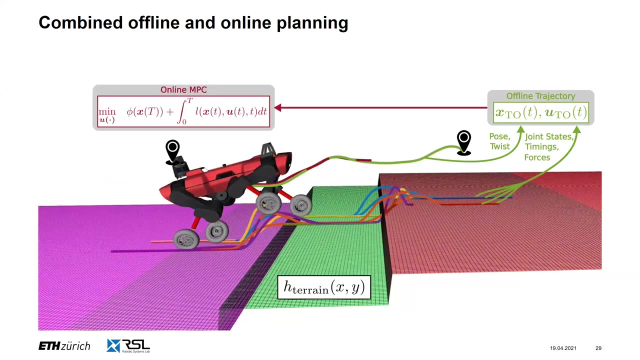 The offline trajectory consists of the robot's torso pose and twist and the legs joint states, timings, when to lift off and touch down and contact forces. Now the robot executes the offline trajectory. One interesting conceptual question raised by our approach is the integration of the offline trajectory given by xto and uto into the MPC. 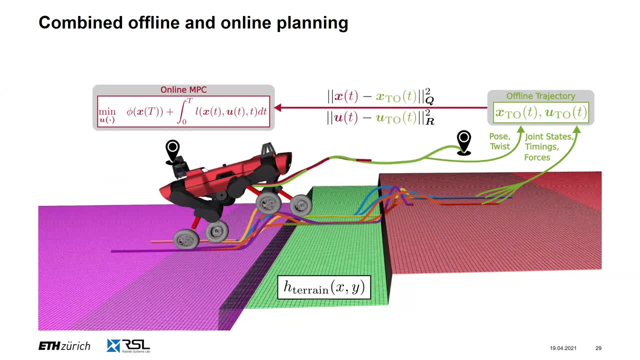 We achieved this by feeding the offline trajectory as a quadratic cost term into the final and time-varying cost, The MPC's optimized control policy. the red U is applied to the robot at each iteration until an updated policy is available. With this framework, the robot executes the motion. 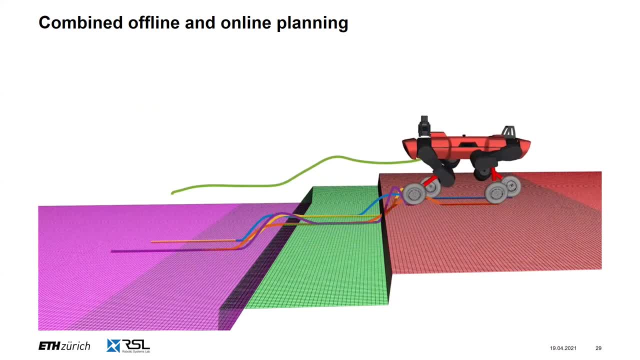 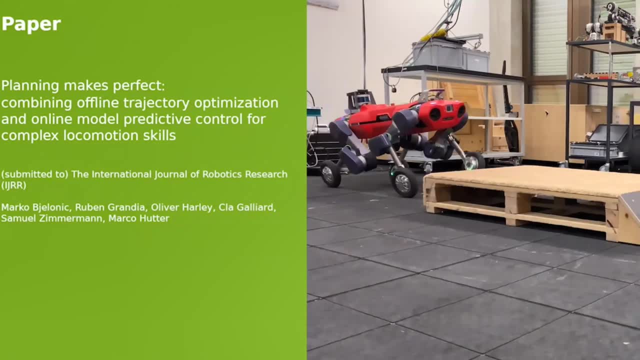 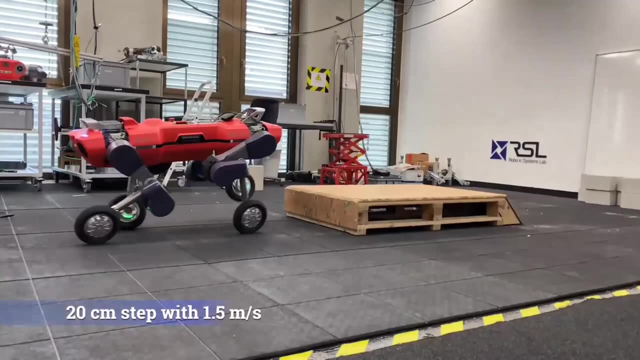 by optimizing online along the offline trajectory and being reactive to unforeseen events. With this combination of offline and online planning, we can generate highly complex and dynamic motions, like turning motions with 4 rad per second, motions over the steps at 1.5 meters per second. 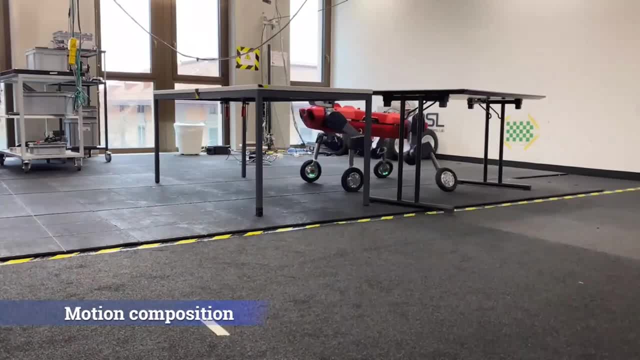 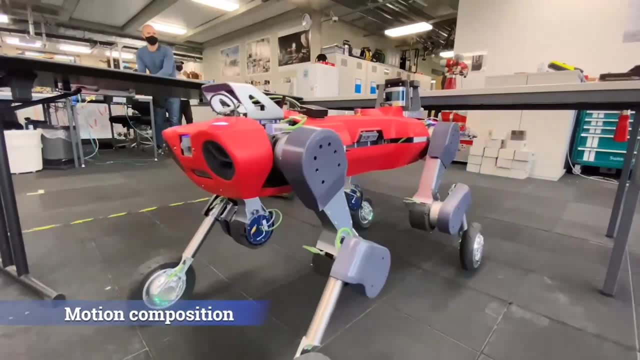 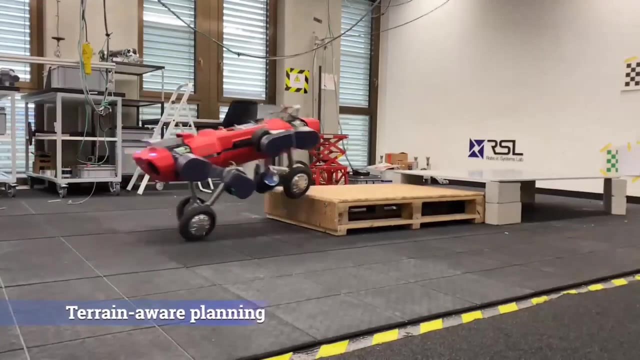 We can compute motions together to achieve even longer motions. These motions are another unique example of how wheels can help to duck down under narrow objects without even stepping and by solely stretching out the robot's legs. Here's another example where the robot overcomes two steps. 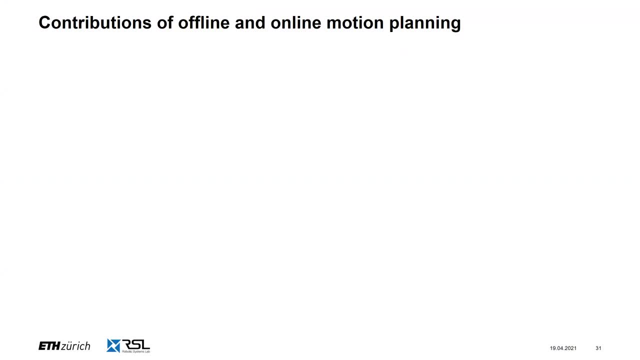 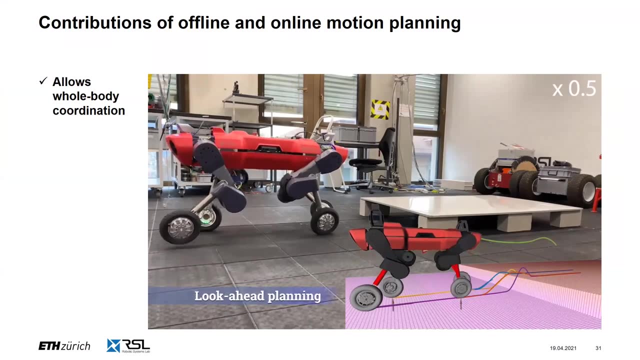 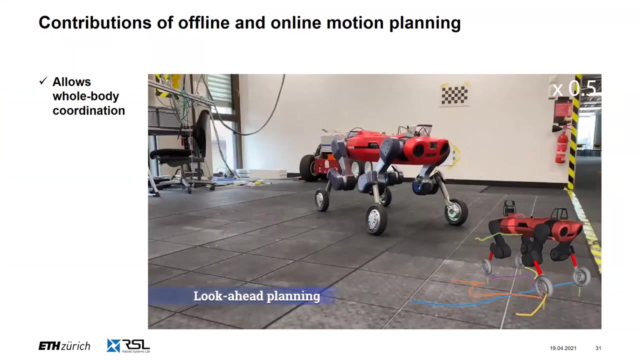 So let me continue by summarizing the contributions of this combined offline and online motion planning. The lower right visualization shows offline and online trajectories while executing terrain aware and highly agile motions Due to the MPC's look-ahead. our approach anticipates future events of the offline trajectory and robustifies them. 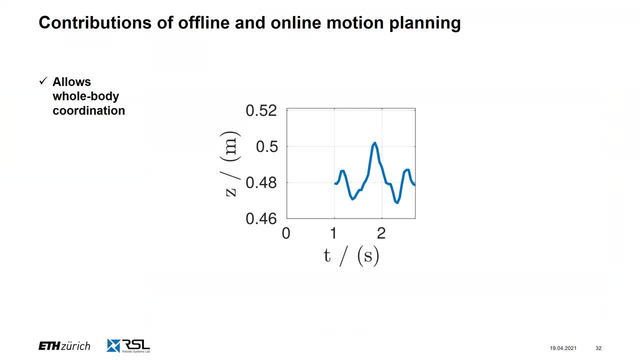 Let's have a closer look at these turning motions. The vertical movement along the z-axis of the center of mass position experiences a discontinuity at t equals 1 second. where the robot switches from repositioning motions to the blue offline trajectory, It can be seen how the MPC's red trajectory anticipates. 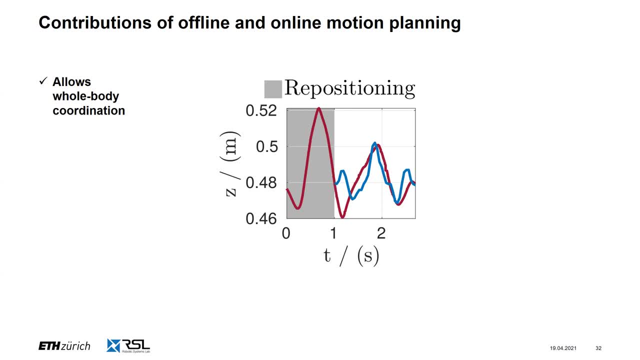 along its receding horizon, the upcoming blue offline trajectory, and finds a solution respecting the whole body state. This plot represents only a fraction of all whole body states tracked through the MPC's cost function. As we can see in this example, the MPC's look-ahead 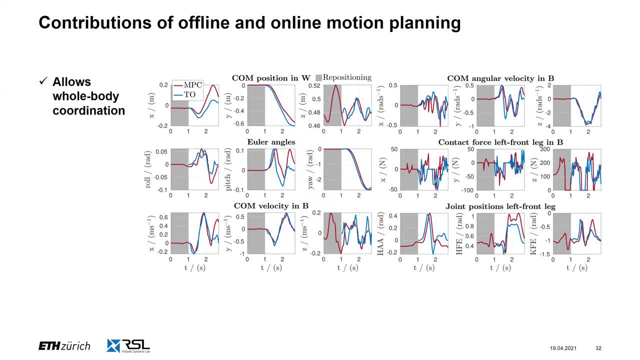 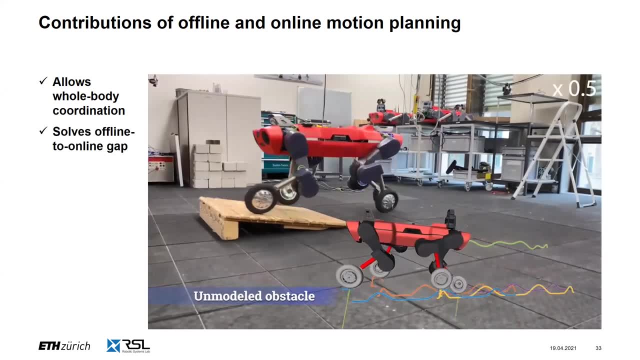 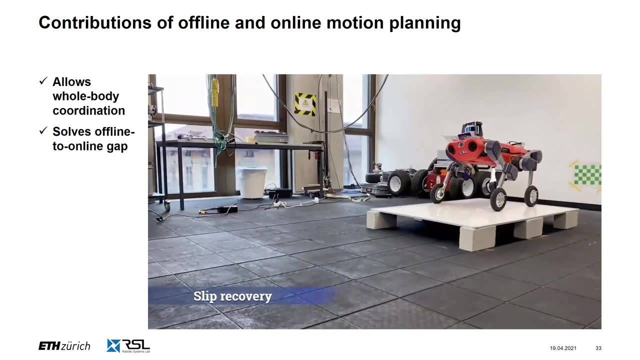 can blend between discontinuous offline motions while considering the future trajectory of 48 degrees of freedom. One of the main challenges of running offline trajectories is the online reaction to our unforeseen conditions. The key to this challenge is our online MPC that robustifies the maneuver to a certain degree. 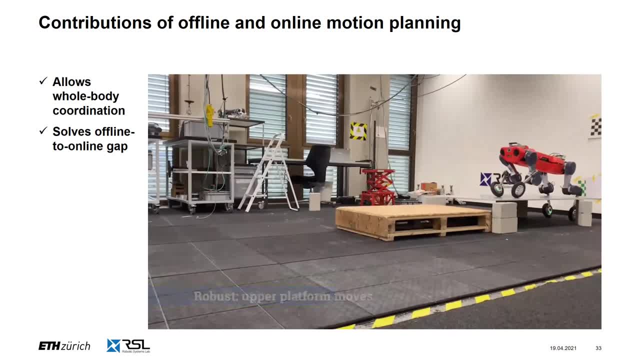 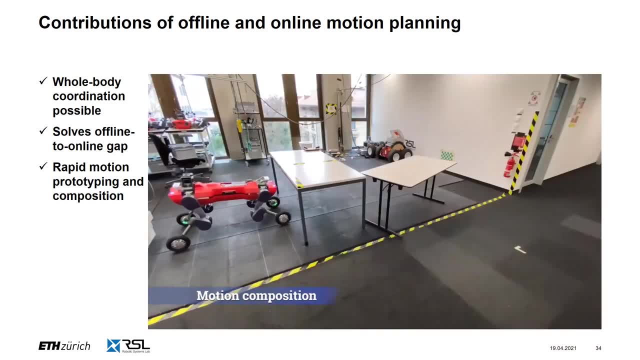 by recomputing solutions on the fly and adding feedback control. With our approach, motion designers can choose their favorite trajectory, optimization routine and iterate over behavioral design offline, without tuning robot experiments, enabling them to author new behaviors in a matter of minutes and as shown here. 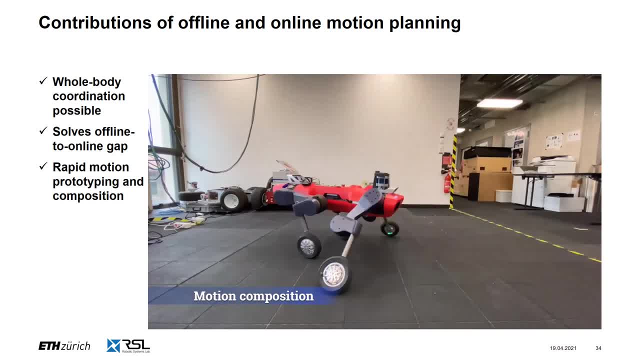 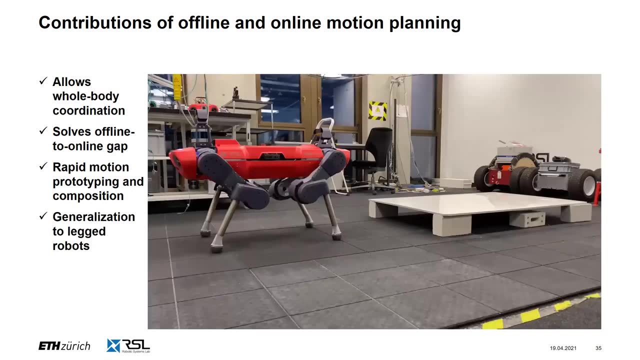 compose multiple offline trajectories out of a motion library into a single maneuver. Throughout this work we generated 99 different offline trajectories and more than 84% can be successfully run on the real robot. We can also perform complex locomotion strategies for robots with traditional legs. 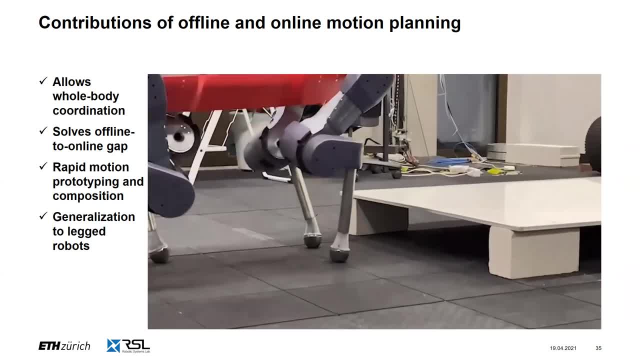 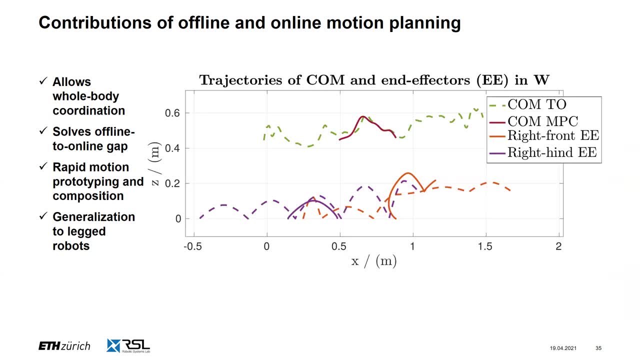 And here's another example how the online planner can react to slippage while anticipating the offline trajectory. Looking more closely from a side view at the trajectories of descent of mass and speed, right legs over the locomotive distance x, we can see how the leg's solid orange trajectory of the MPC 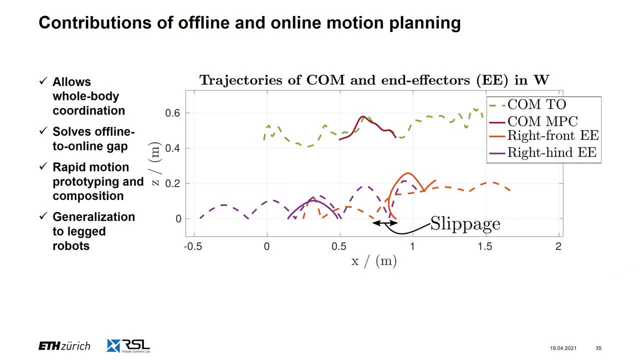 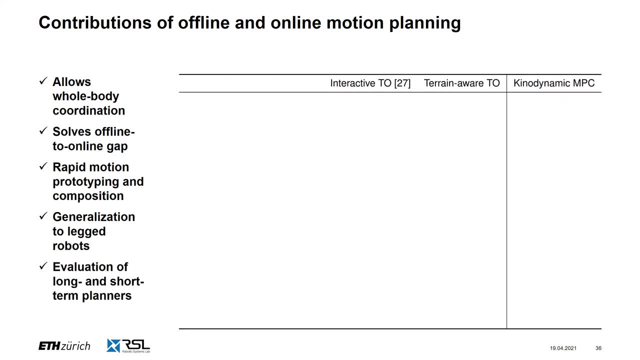 finds a solution that guides the leg back to the dashed offline trajectory despite the slippage, And the robot successfully finishes the motion. For the offline computation of complex trajectories, we exemplary use two trajectory optimizations. Our framework can be combined with other algorithms. 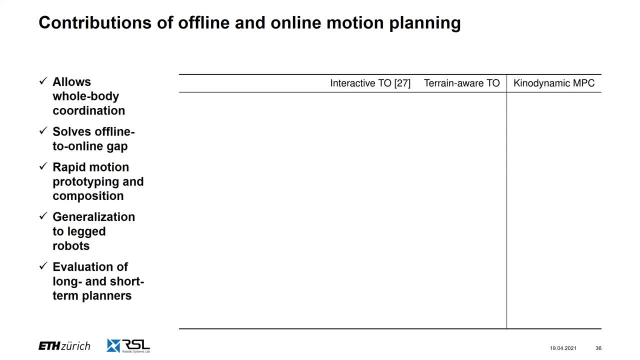 providing whole-body trajectories. In contrast to the online motion planning, the two trajectory optimizations do not allow for clear evaluation, since each algorithm achieves maneuver for a different set of tasks. For example, the interactive trajectory optimization integrates a user-guided interface and the centroidal dynamics model. 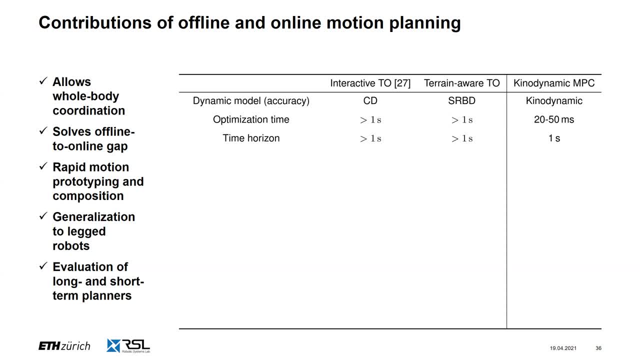 which considers the leg's inertia. On the other hand, the terrainable approach focuses on motions over non-flat terrain with a simplified single rigid body dynamics model, while adapting gait timings. Both trajectory optimizations rely on the online tracking approach of the MPC. 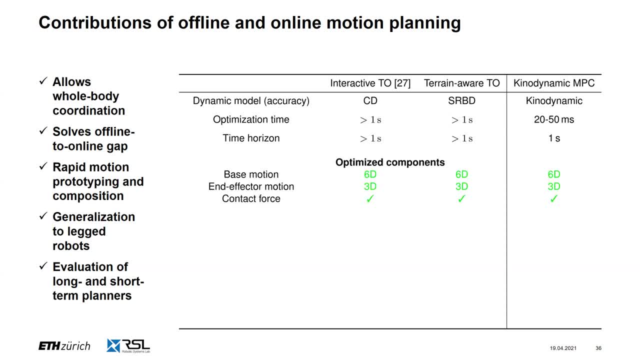 All of these approaches solve the problem as a single task while simultaneously considering the torso and end effect of motion. The terrain-aware approach does not consider the joint kinematics of the robot, but that allows for optimization of gait timings On flat terrain. 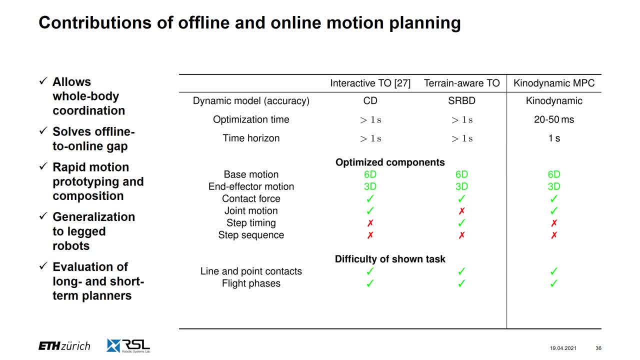 these approaches can execute any set of gait patterns. Their interactive trajectory optimization is, in the current form, not used for non-flat terrain but in theory could be extended. Since the terrain approach does not include the kinematics of the robot, it requires a heuristic to estimate the wheel's rolling direction. 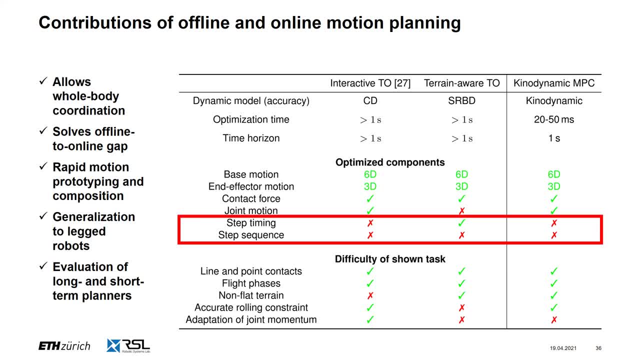 There is one problem with these offline trajectory optimizations: They struggle to optimize the gait sequences and timings, since they are highly dependent on the initialization. Adding these optimization variables to the problem would require, for example, mixed integer programming, which is a hard problem to solve. 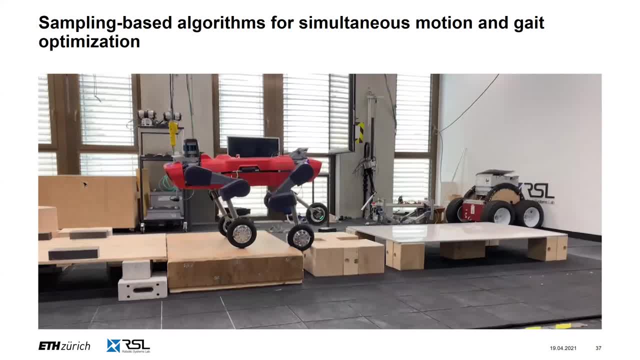 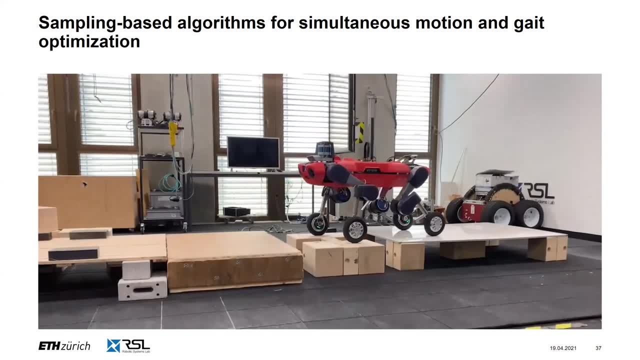 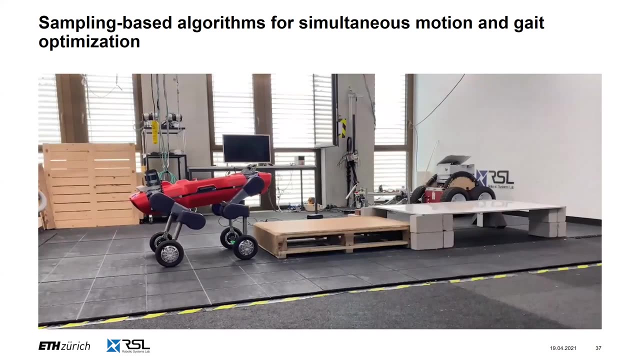 One way to solve this is to use sampling-based planners for the offline part that simultaneously optimizes kinematic trajectories and step sequences, as shown here, over stepping stones and, as we will see in the next example, again over these double steps. So what we actually do here is having a sampling-based approach. 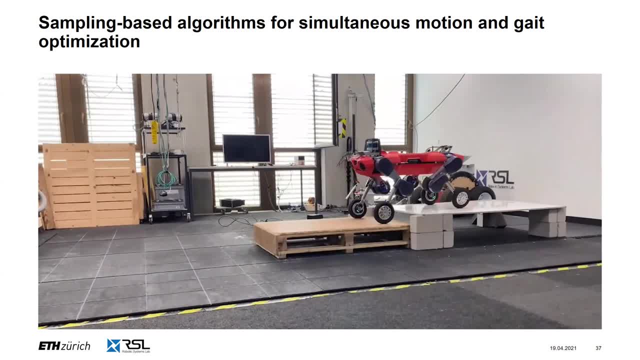 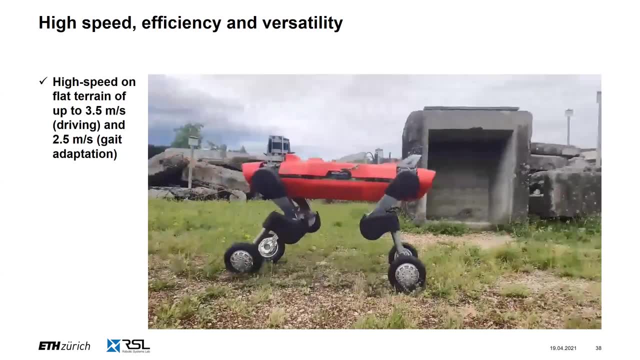 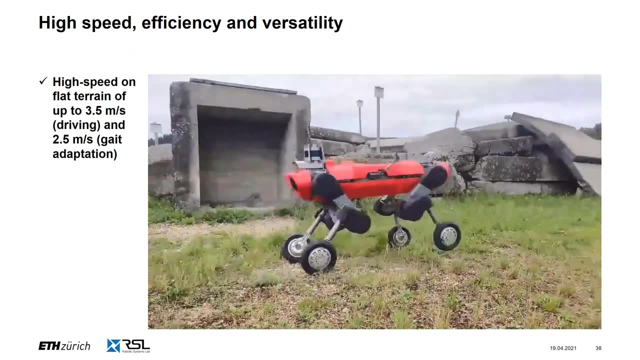 that finds different ways of adding the gait sequences and gait timings to the optimization program. In the following we address the speed and efficiency aspect of wheel-legged robots. Our wheel-legged robot can achieve a higher speed than its traditional legged version. 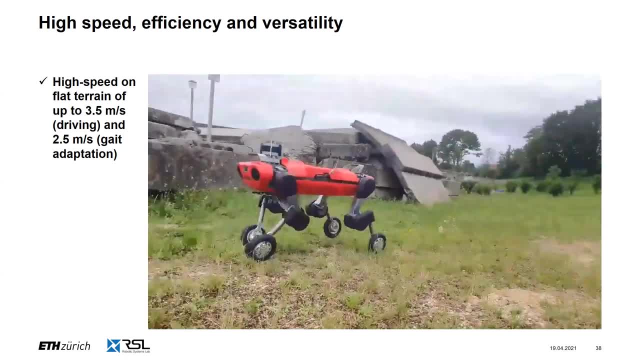 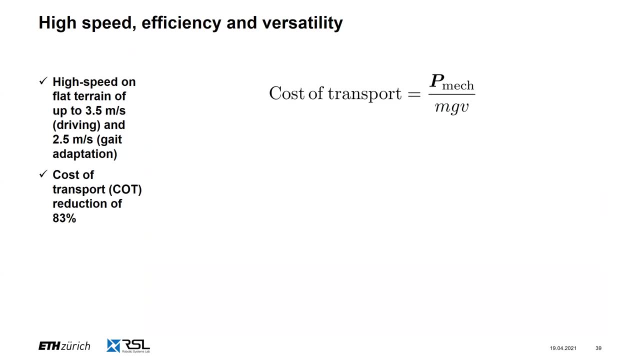 which is mostly limited to speed and one meters per second, while our speed in theory, is only limited to the wheel's maximum speed and radius. To compare the cost of transport of legged robots, gaits here in blue- and wheel-legged robots. 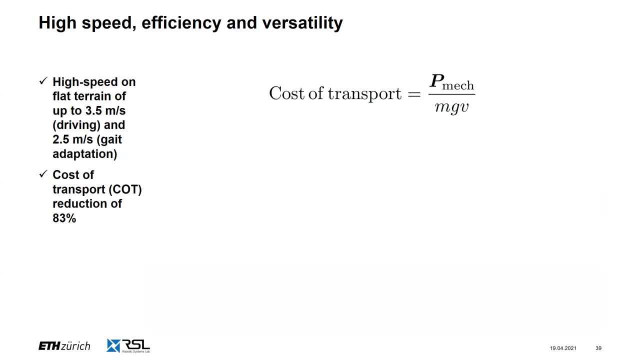 to address the energetic efficiency of hybrid locomotion, we compute this dimensionless cost of transport, which is the mechanical power of the system divided by the mass m, gravitational acceleration g and speed v of the robot. If we compare now the cost of transport: 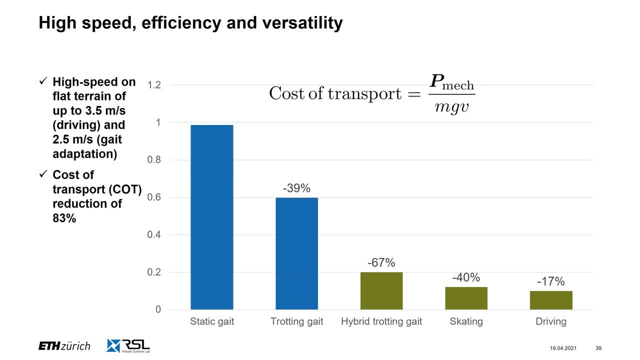 of legged robots gaits here in blue and wheel-legged robots gaits here in green. we can immediately see how these hybrid gaits lowered the cost of transport drastically. For example, pure driving reduces the cost of transport by 83%. 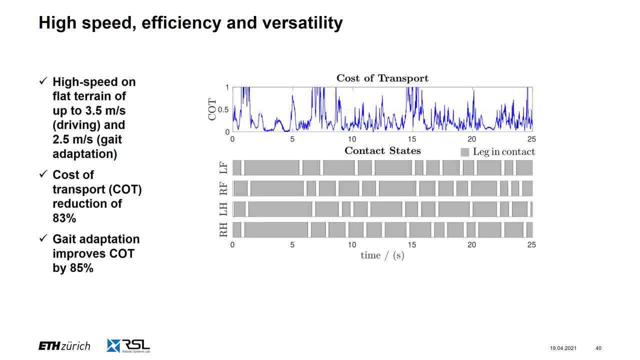 compared to traditional trotting gaits. Here we see a time snippet of the cost of transport and the contact states when the robot adapts its gait sequences. If we look more closely at the contact states, we can see that the robot executes pure driving motions. 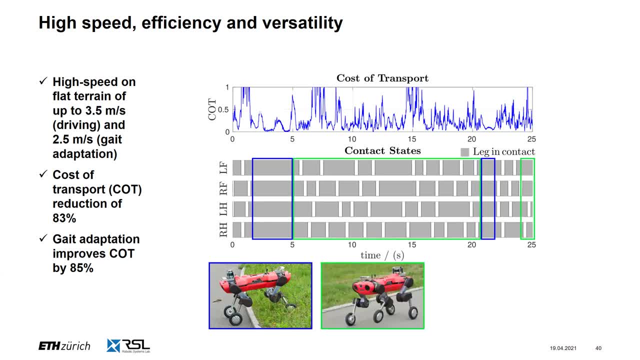 in these blue areas, Since the robot has non-seeable wheels. the robot executes aperiodic gaits like a hybrid static gaits in these green areas, lifting one leg at a time, and a hybrid trotting gaits in the red areas. 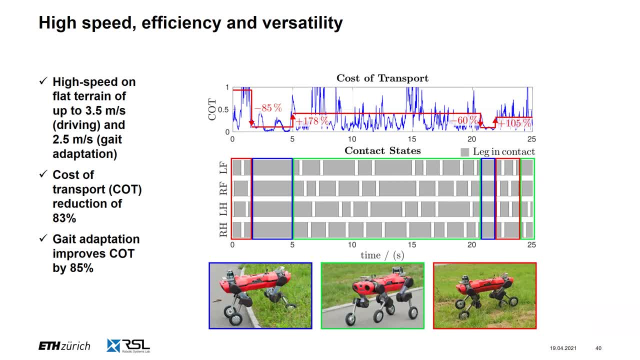 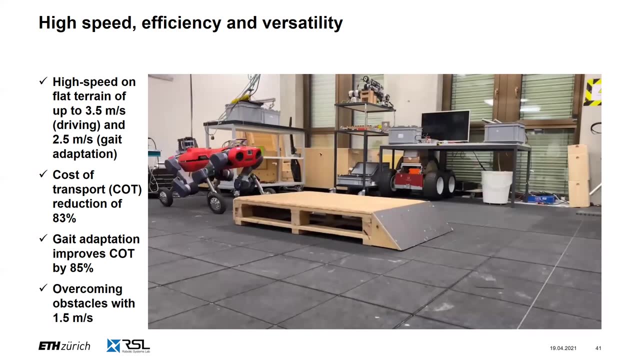 The cost of transport plot in the top reveals that with our online gait adaptation, we can automatically switch between aperiodic gaits and pure driving motions, reducing the cost of transport by up to 85%. Adding wheels to legs does not just increase the speed and efficiency. 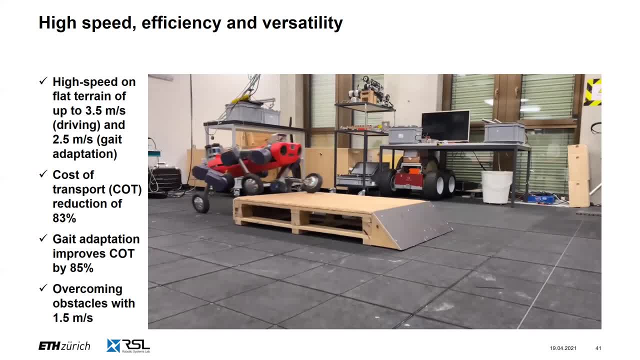 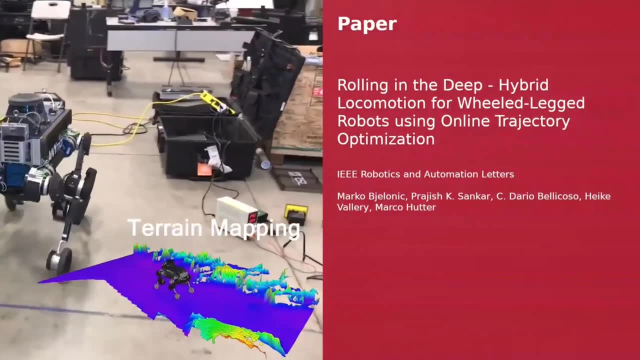 on flat terrain, which is probably intuitive for everyone here, but this multimodal robot achieves even fast motions of up to 1.5 m per second over challenging obstacles. We also validated the decomposed motion planner and an early version of our roller-walking robot. 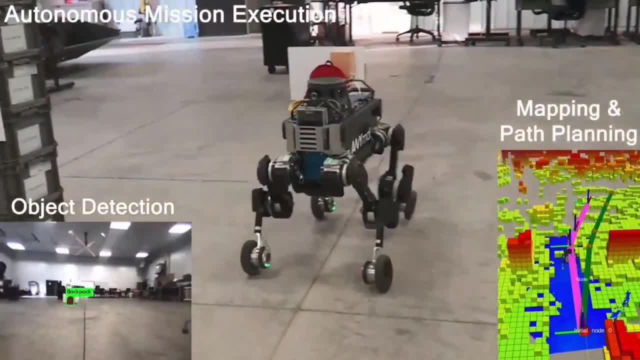 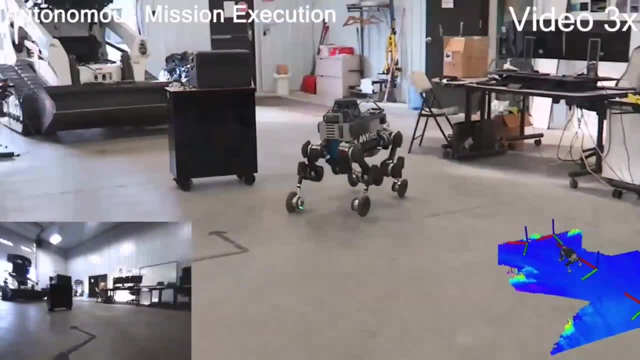 during a real-world competition At the DARPA Subterranean Challenge. the robot rapidly mapped, navigated and explored dynamic underground environments. Here it can be seen how the robot generates an elevation map and incorporates object detection, SLAM and navigation algorithms. 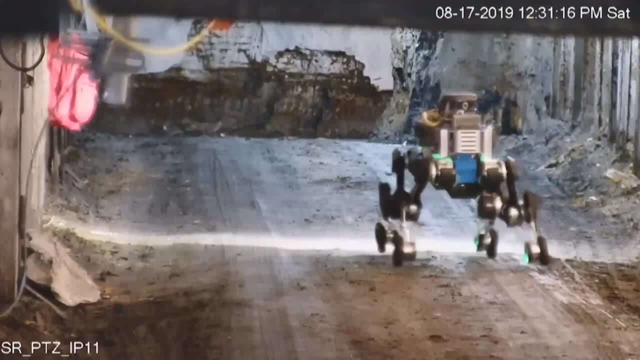 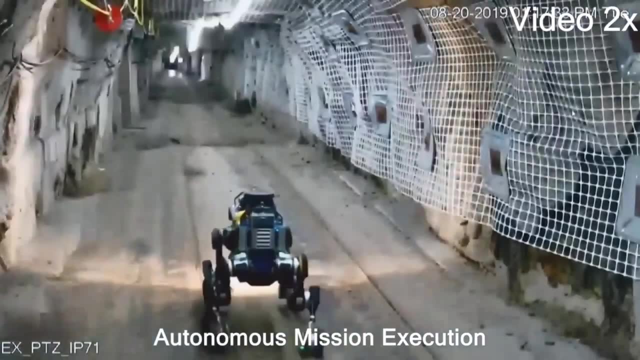 At the tunnel circuit in Pittsburgh. the wheeled version of Animal achieved more than double the legged robot's speed, and the robot scored important points for the Cerberus team. As you can see here, the terrain was a challenging, multi-terrain. 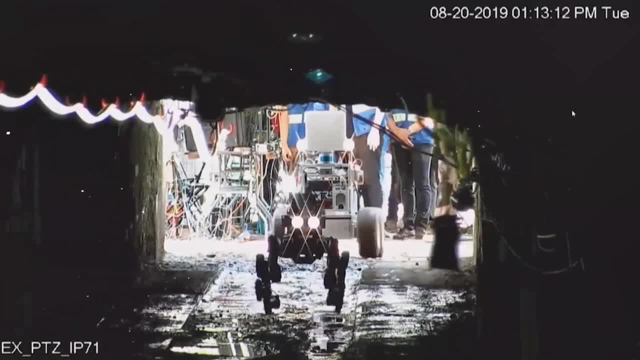 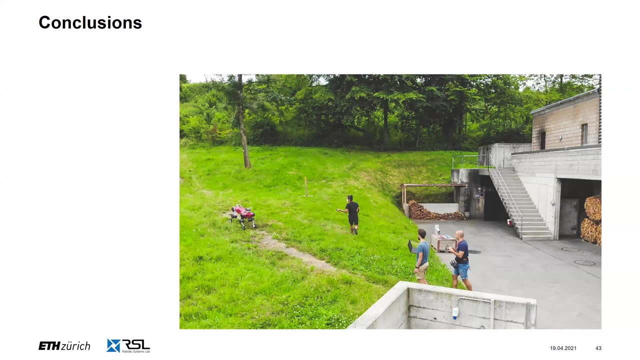 and the decomposed motion planner had difficulties to traverse the terrain. The lessons learned from this competition paved the way towards more robust single-task planners. With this image from Wangenlander ARA, I would like to conclude this presentation. Throughout this work. 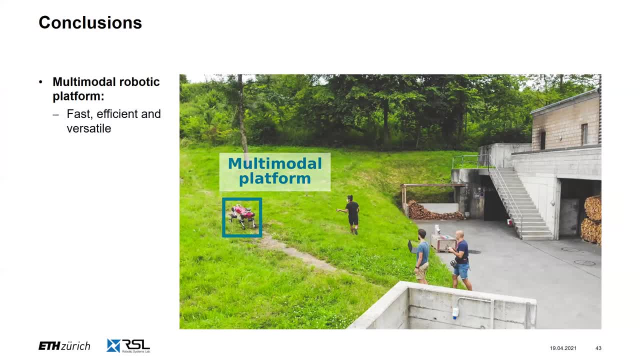 we developed a novel multimodal platform Achieving fast, efficient and versatile locomotion. we explored two different online planning algorithms that generate fast solutions over relatively short horizons And, due to these fast update rates, we can add feedback control that diversifies the motions. 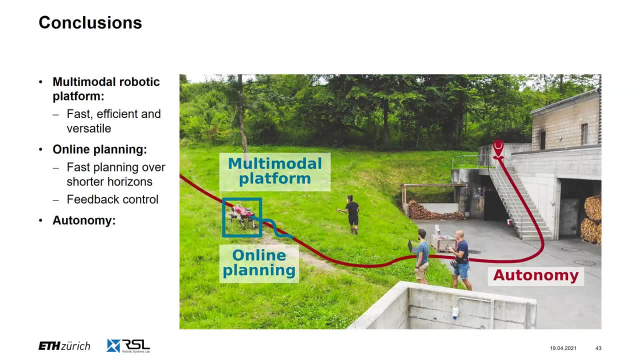 Throughout the DARPA competition. we integrated higher-level autonomy to the robot, like SLAM, local and global navigation routines and subterranean exploration methods. Finally, the combination of offline and online planning achieves complex motions over obstacles and at the robot's limits. 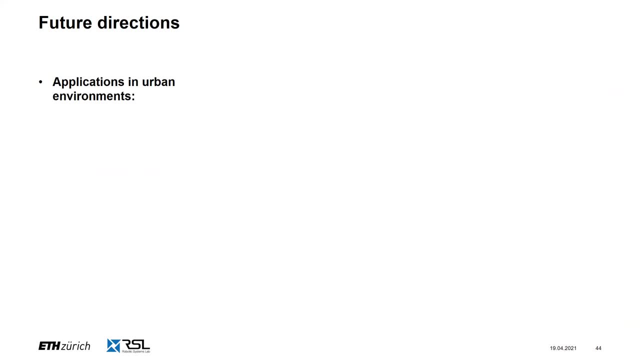 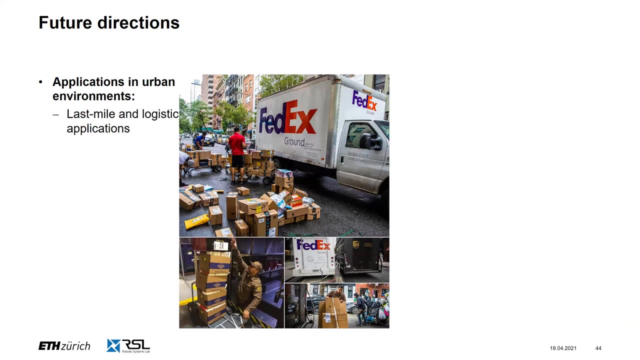 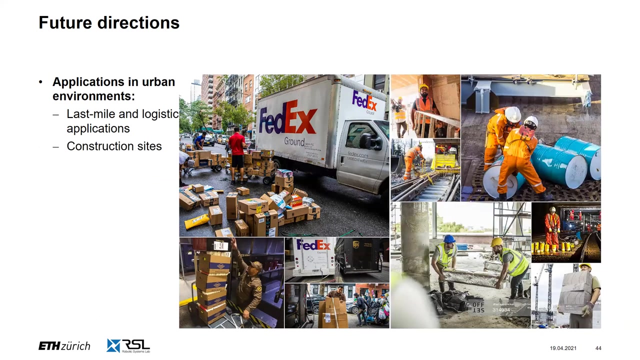 Let's have a closer look at the future directions of this project. For the last mile delivery problem in urban environments, we foresee that weed-legged robots must shift the share from human-piloted and fuel-powered vehicles to electric, small-scale autonomous solutions. We also envision transporting tools and materials. 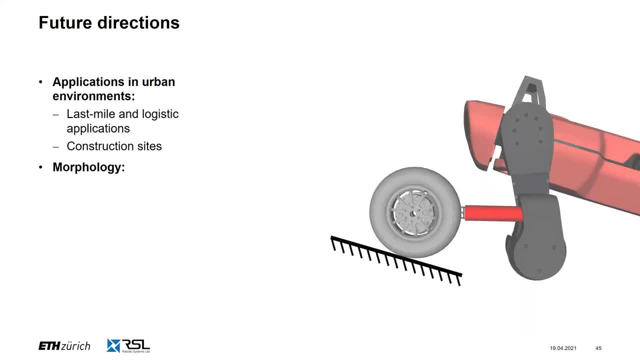 in industrial and construction sites. Optimizing the morphology of a weed-legged robot is a fascinating avenue for future work. In this work, we merely added the wheels to animals' feet, but this doesn't allow for pure driving motions while turning, which would be essential for higher speeds. 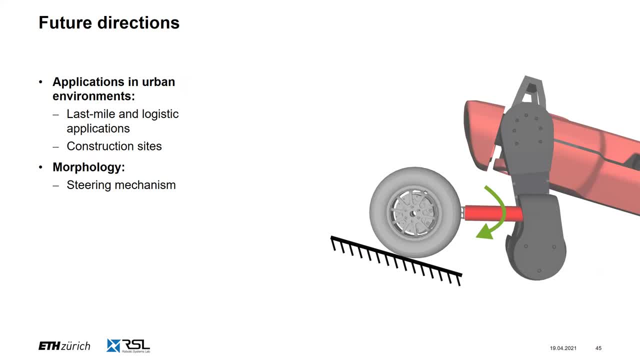 Adding a steering mechanism to the wheel improves the robot's mobility, but comes with additional hardware complexity. With a novel leg design that is inspired by hexapetal robots, the robot can control its orientation or position on the ground without adding hardware complexity For this purpose. 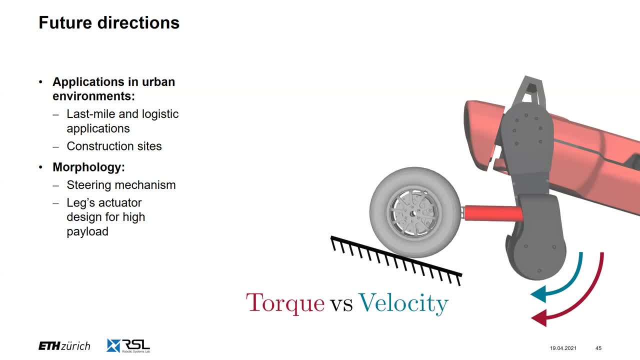 we merely have to rearrange the legs first actuator. Increasing the robot's payload capabilities could open further markets in many industries. In theory we want actuators with high speed and torque, but in practice a trade-off needs to be found for electrical motors. 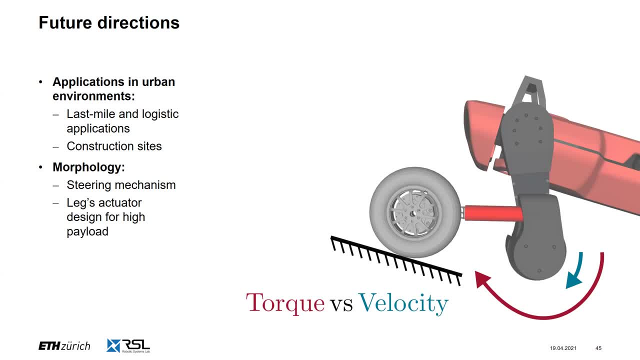 Such a trade-off is not required for weed-legged robots, since their speed comes through the wheels and allows for actuators in the legs with higher torque and lower speed requirements. To make the system applicable for the last-mile delivery, we need to further research and improve its autonomy. 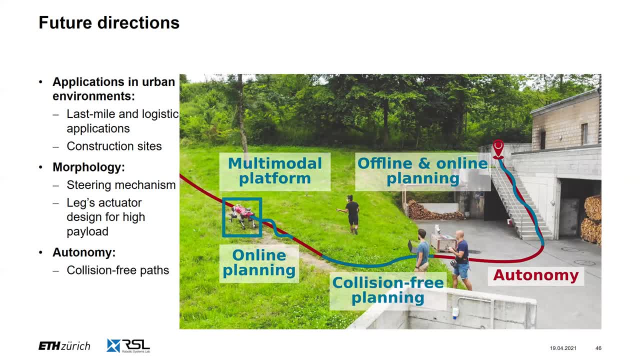 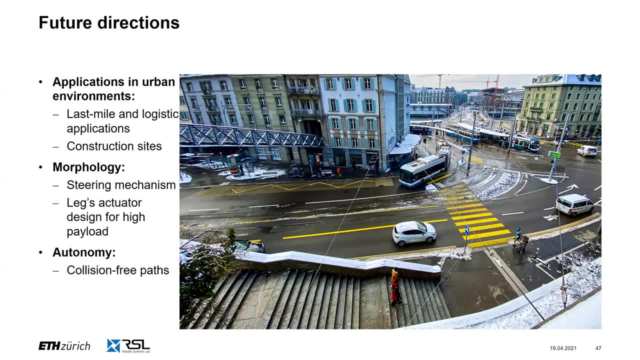 where we target navigation in urban environments with moving obstacles like humans, cars and other vehicles, thus requiring collision-free planning. But if we look more closely at this particular scenario, it is a difficult problem to understand and plan a path in such dynamic urban environments. 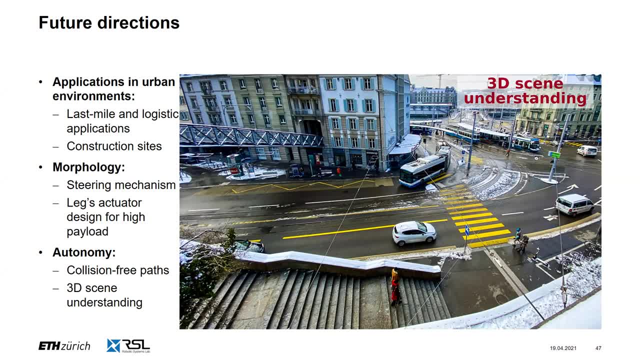 Thus, the understanding of the 3D scene becomes crucial and requires the identification of traversable terrain and navigation goals. Based on this 3D scene, we need to plan a safe navigation path to the target location, considering the robot's unique mobility skills. 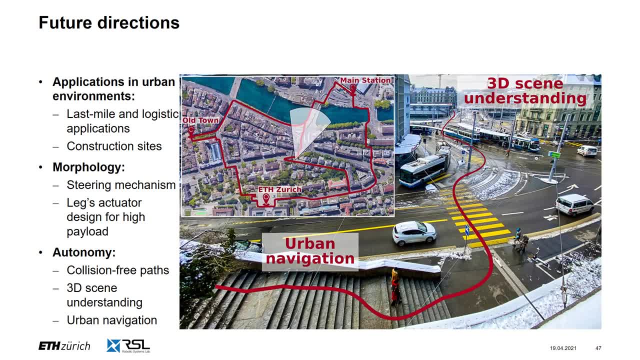 and available maps of the environment. One might imagine a day when our robot is required to autonomously navigate from the old town of Zurich to the main station or university incorporating all of these aspects. With this, I come to the end of my presentation. 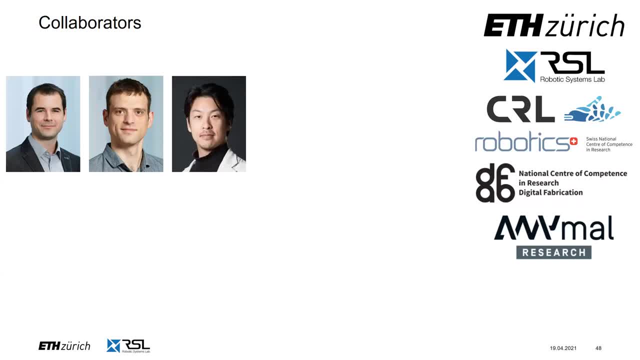 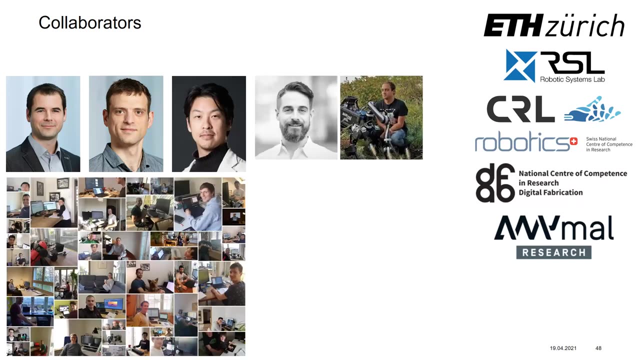 I would like also to thank my collaborators and my advisors, Professor Marco Hutter and my two co-examiners, Professor Steljan Koros from ETH Zurich and Professor Sambe Kim from MIT. I benefited from the great environment at ETH Zurich and the talented contributors at the Robotics Systems Lab. 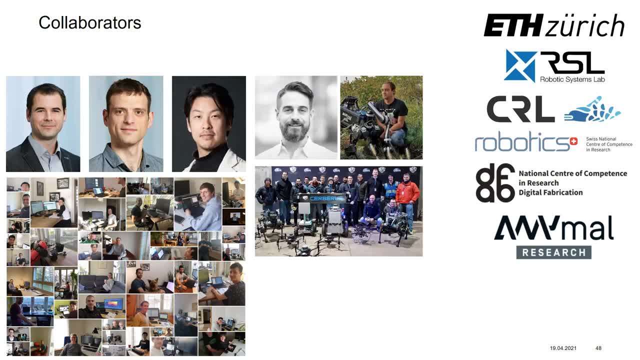 that I would like to show here. I also would like to thank the DARPA team for the opportunity to learn more about real-world applications. although it was mostly hard work, from time to time we managed to have some relaxing team-building moments, as shown here at Lake Tahoe. 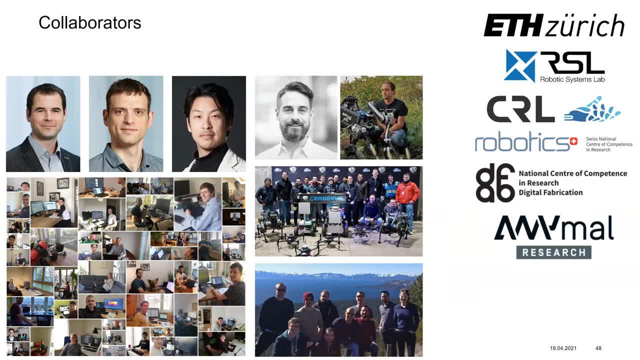 Now the dancing motions of the unmuted video on the next slide was also created with our offline and online motion planning approach, And then at the end of the video we show some new developments recently that we managed with reinforcement learning algorithms. Thank you for listening. 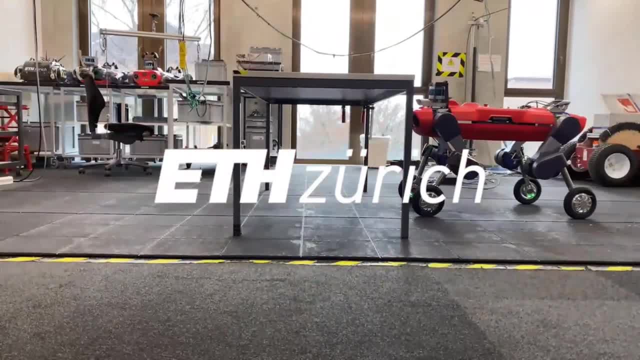 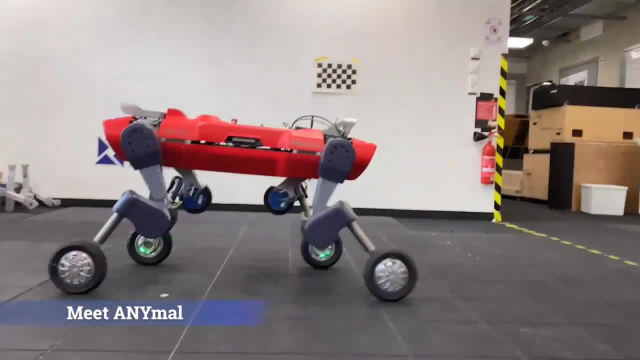 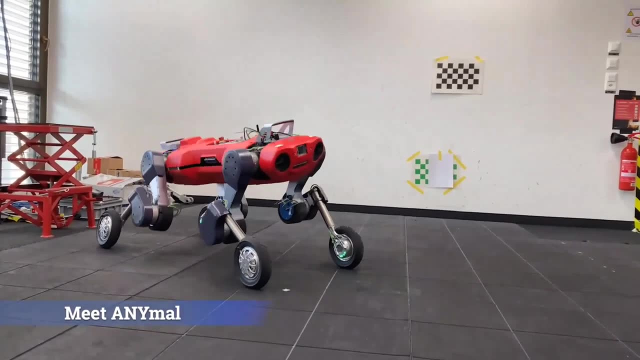 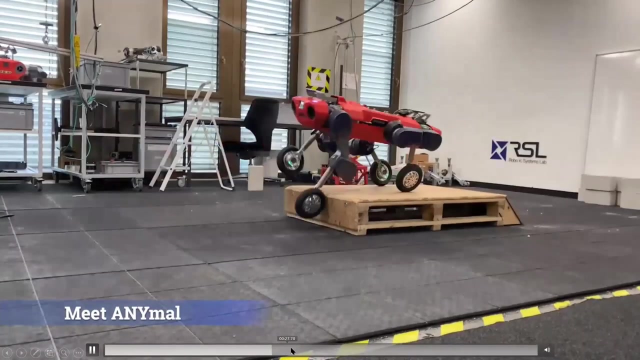 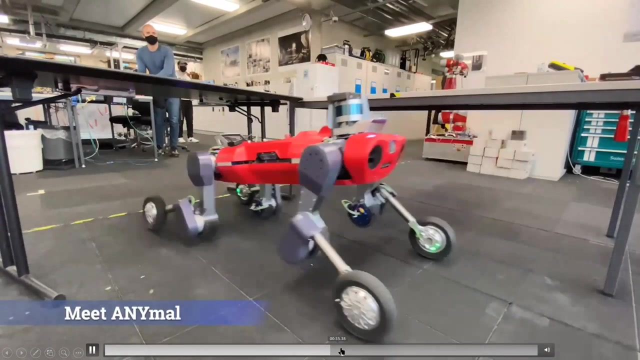 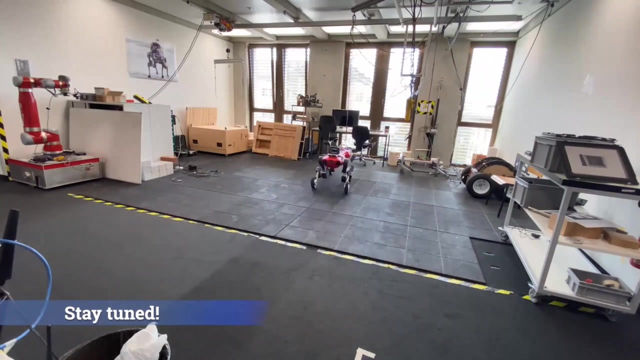 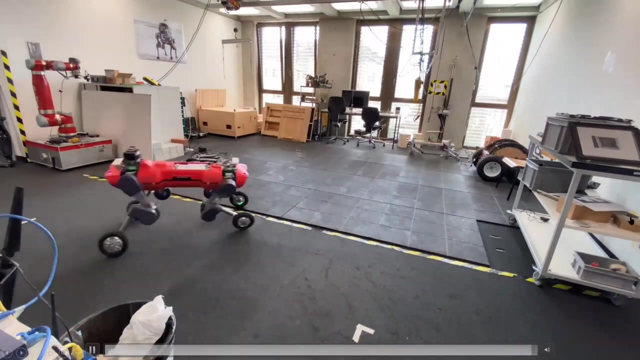 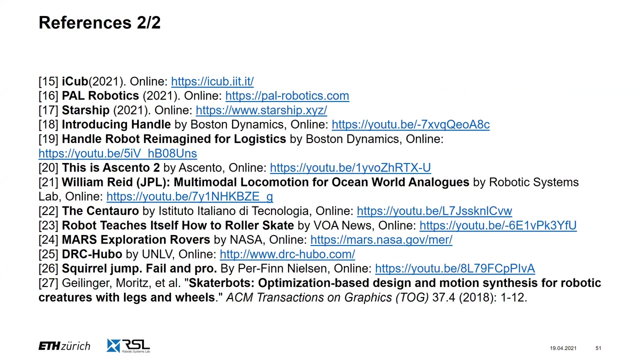 Thank you. Thank you, Yeah, so I'm happy to answer now all the questions here. It's just some references that I used during this presentation. Thank you very much, Marco, for the great talk. Are there any questions from the audience? 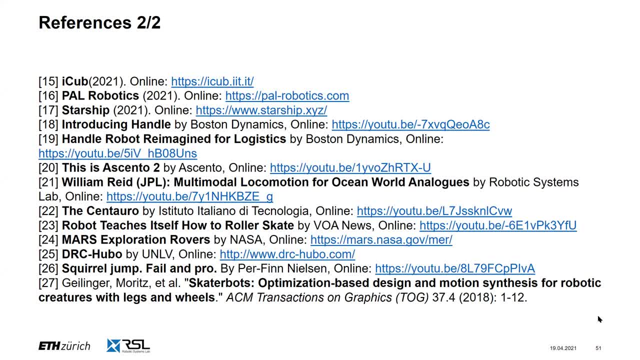 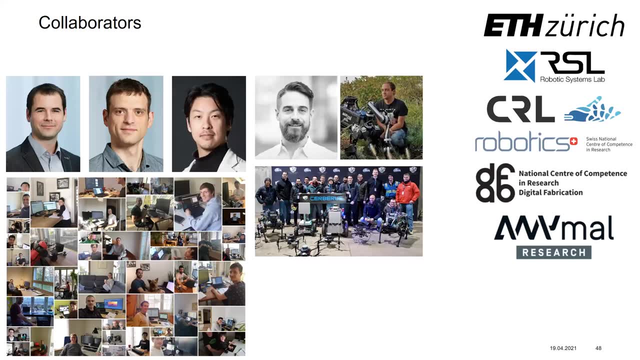 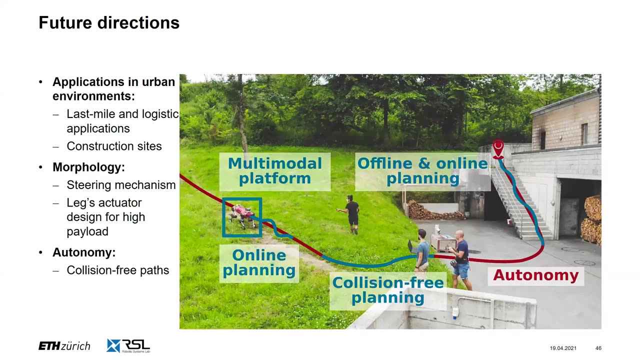 If so, please unmute yourself. Hi Marco, Hi Marco, Here's Julia. Hi, I have a quick question to this combination of offline and online planning. Could you talk a little bit about the timescales? I think you might have had them in one of the table. 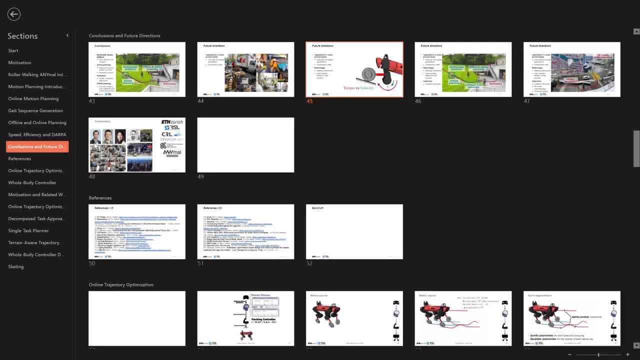 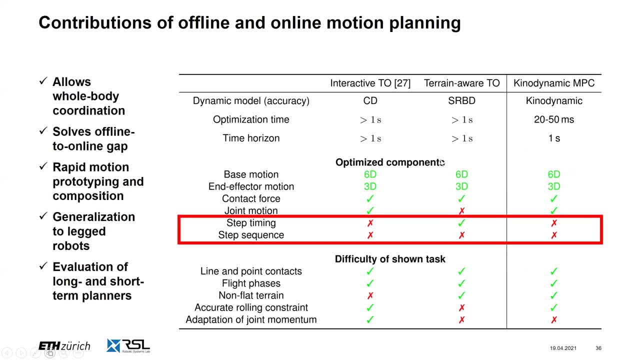 but specifically the offline planning. How much time do you need to plan in advance when you combine it with online planning, And what is the basis for your planning? Like this terrain knowledge? where does it come from? Yeah, So the first question here can be maybe answered. 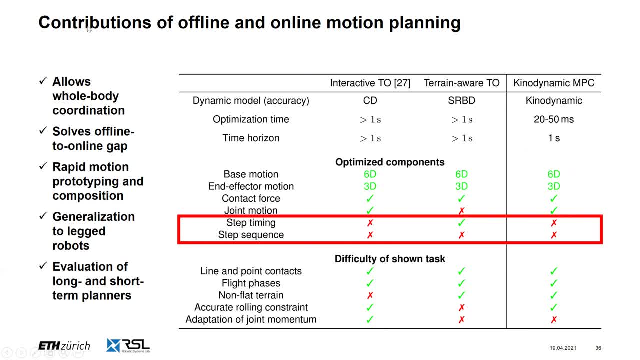 with this slide. So you see this interactive TO, which is the interactive trajectory optimization or this terrain aware trajectory optimization. The optimization times really highly depend on the task that we have to fulfill. But if we, for example, for this double step going up, 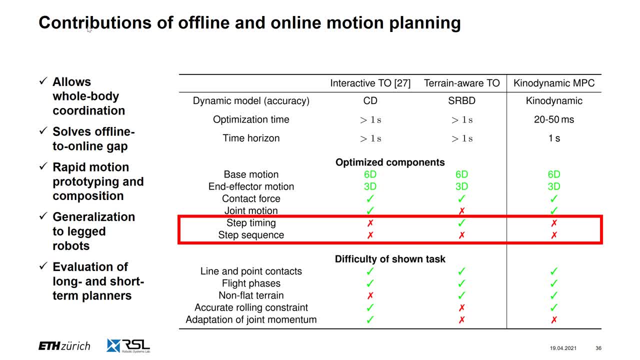 or going up a step and going down. we need, for example, to optimize such emotions up to like 30, 40 seconds, And the time horizon also varies really depending on the task, But we had time horizons of up to seven seconds. 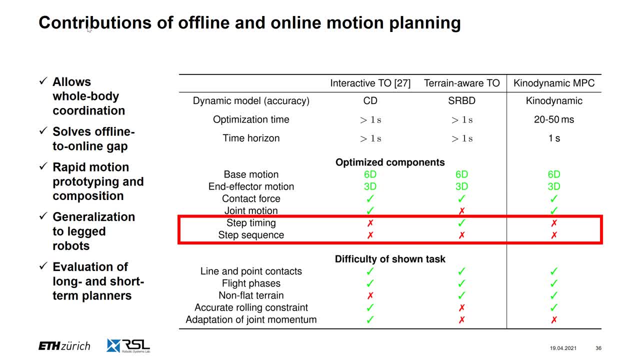 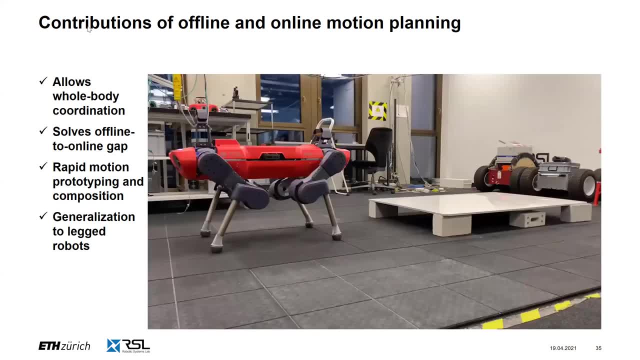 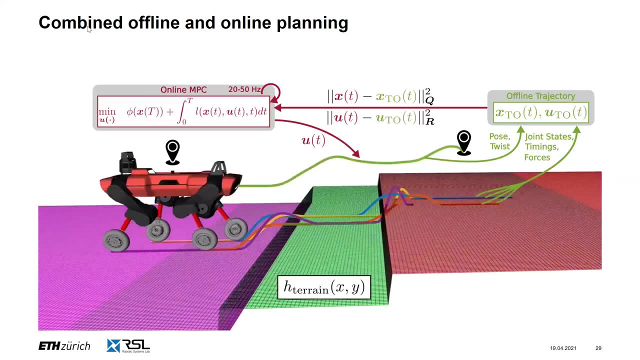 For going up the two steps. I think the time horizon was about three seconds. And for the second question that you asked, the representation of the terrain can be explained best In this slide. So what we actually have here for the terrain is this height map. 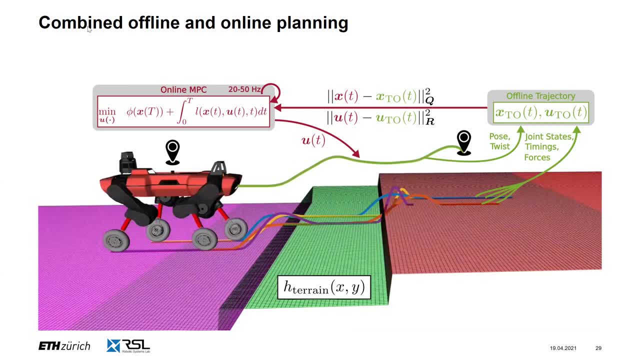 And the height map is actually just a 2.5D representation of the terrain, So you can imagine we have these kind of grid cells for each position in the world frame that gives us a height And we use this in the trajectory optimization. 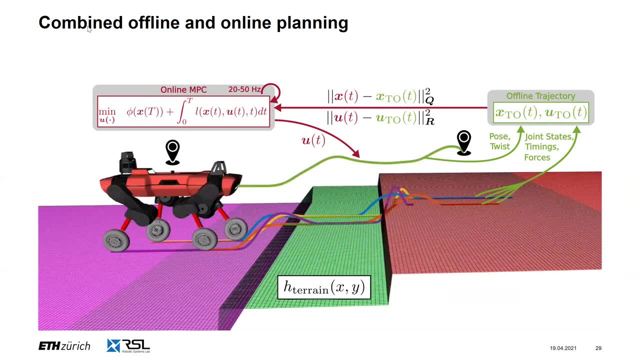 Cool thanks. Maybe a related question. I just see in the chat from MP He asks: in research, it seems that online planners are becoming much more complex, nonlinear and therefore slower Rather than a fast, and it says more than 400 hertz. 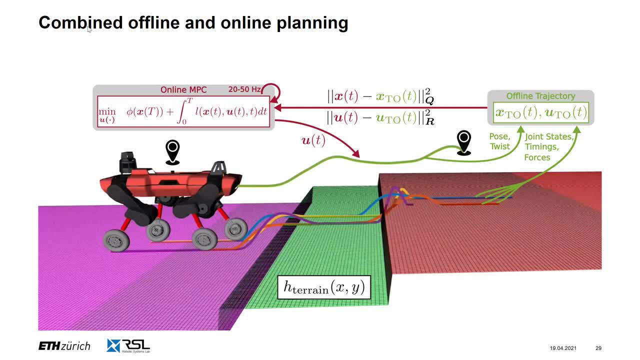 simple model-based planner that guarantees balance while driving. MPCs now are considering full kinematics or collision avoidance, et cetera. This is apparently fine in a lab setting, although do you think these methods are robust enough for real industrial settings? How easy is to justify such low rates? 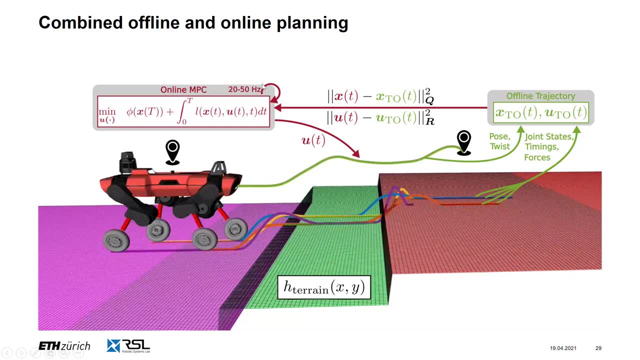 So actually I'm already on one of the great slides to answer this. So our online MPC runs at like 20 to 50 hertz And we found in our lab settings and also in all the competitions that we are facing, that this is. 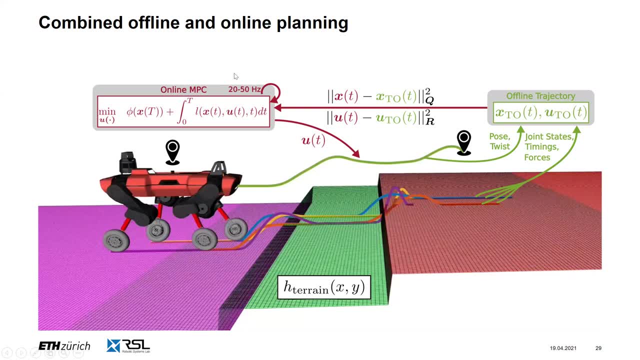 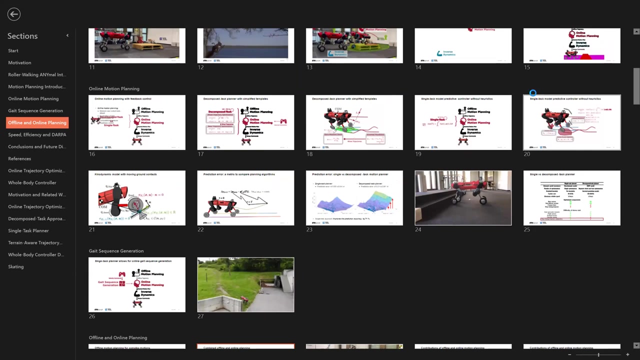 again a lower bound to what is actually feasible to run on the real robot with feedback control. So everything that is in this timescale can be run on the robot successfully And actually our online MPC. let me change the slides for that here. 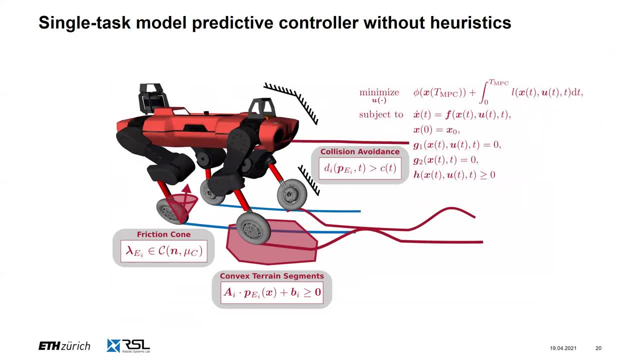 As you can see, in our MPC we almost include all the properties from collision avoidance, friction, cone, convex, terrain segments. It uses the full kinematics and a single rigid body dynamics. Recently some of my colleagues also were running this with full rigid body dynamics, which 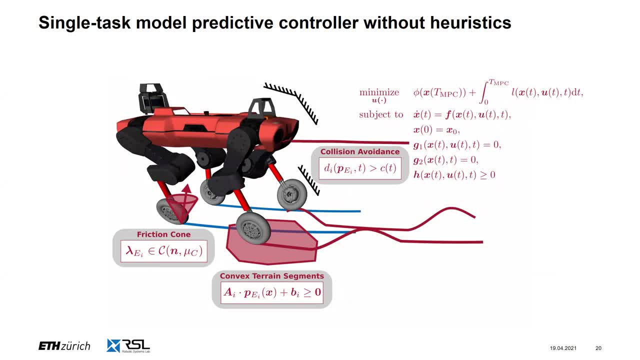 means you also include then the inertials of each of the links of the legs. So there we are actually running the MPC on the real robot, And this is the only limitations that we are having with such an approach is that we can only generate 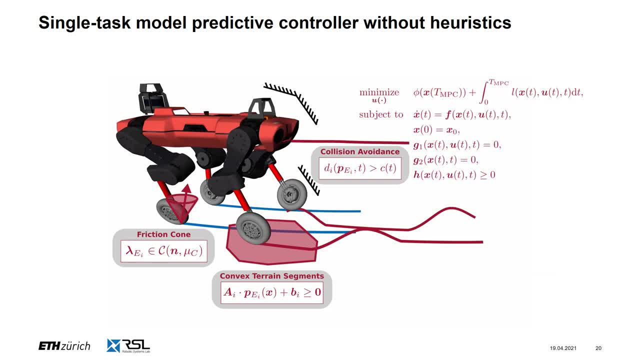 trajectories over like one or two seconds horizons, And everything that considers a longer time horizon then needs to be computed offline. But for the daily operation in our labs this is feasible to run, And I foresee that there are many more ways to make the optimization problem even faster. 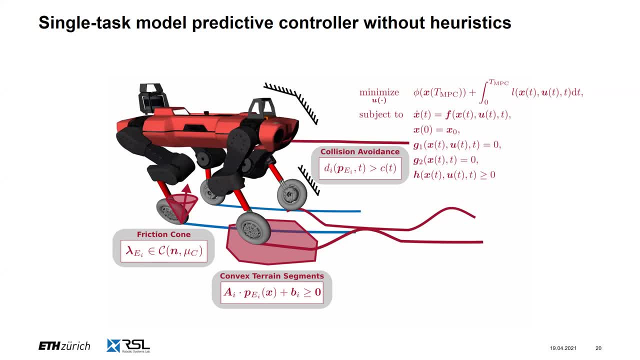 A colleague of mine replaced now our solver that we use for this MPC, which is until now a DDP-based optimization, with an SLQ algorithm and replaced it with multiple shooting algorithms where the same optimization problems was able to be parallelized And we achieved then update rates. 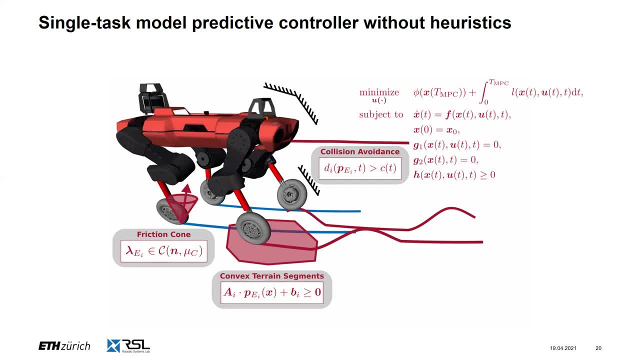 of the same complexity of up to 100 to 200 hertz. So I think there are always ways to improve. Nevertheless, I think this offline planning will always become important, even in the future, if we have more compute, because then we really would like to tackle even larger problems. 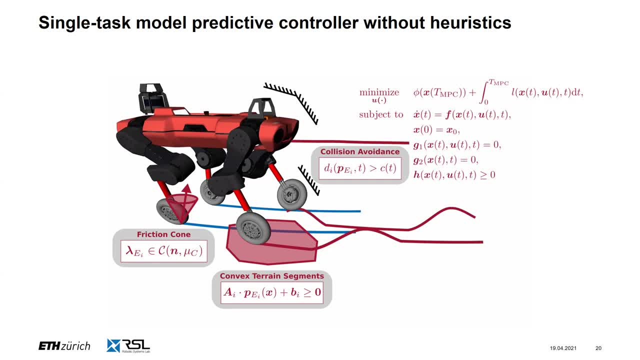 of considering climbing a wall where we have to consider more and more constraints, And I think with every improvement that we make, we will be able to accomplish more tasks than, in the end, Great. Are there any other questions from the audience? Actually, I have one. 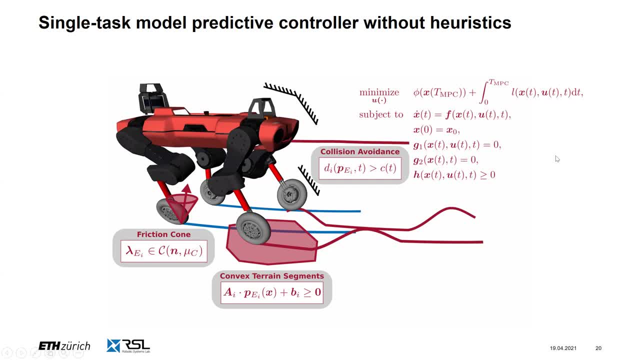 So in your bio you said you are a future entrepreneur. Do you want to talk a bit more about that? I saw you last mile delivery problems in the motivation You're developing these robots. I guess Yes, So I'm going to stay also in the lab. 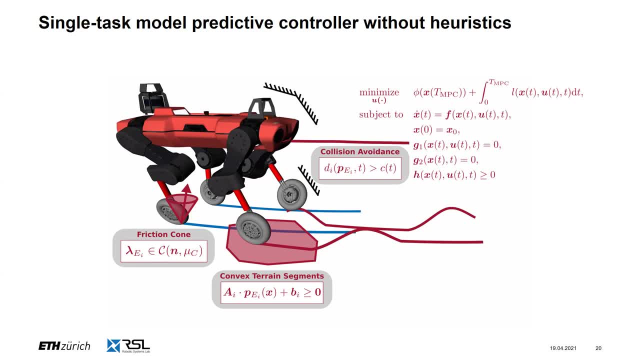 and I will try to pursue to make something more concrete out of this idea. So for that, we would like to now go a little bit more into applications and try to apply this robot together with customers to see what are the needs and where such a platform could be useful. 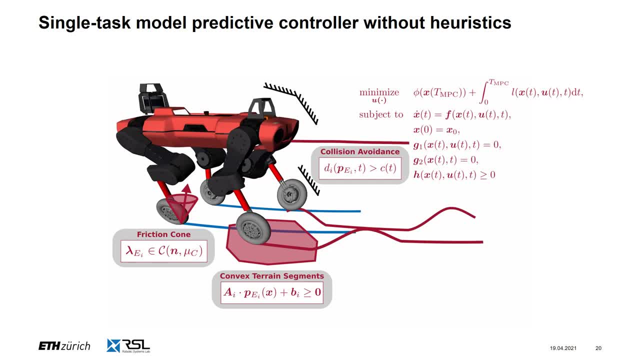 On the same time, our lab is working on new robots with higher payload. It would be also perfect for such kind of applications. Yeah, that's a very cool problem. For instance, you could also use current transportation systems where you can put robots in there. 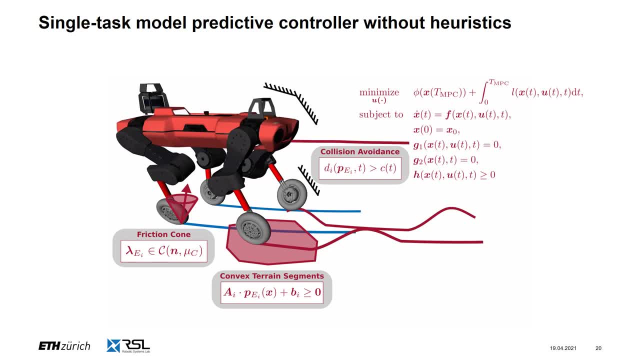 Yeah, Walk to the last mile. It's a very cool problem. Yeah, Yes, that's why I'm also excited about this whole navigation problem. Also, we could see in the last two or three years, especially also with the development of reinforcement learning algorithms. 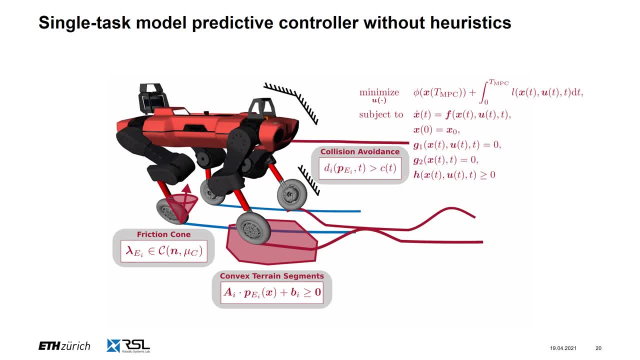 that make these robots really robust. we can see that more and more the basic locomotion concept over stairs, steps and flat terrain is going to be kind of solved. But the next problem is really for such robot: how can it navigate in cluttered environments? 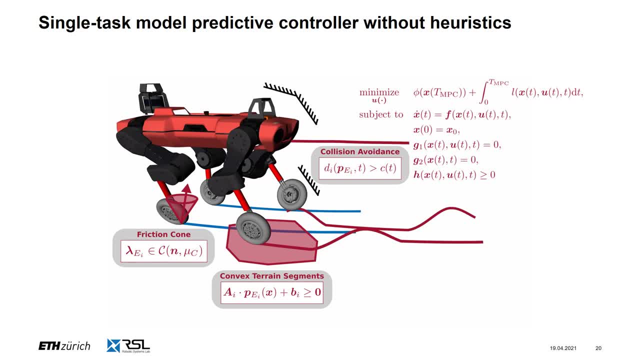 in an urban environment, consider moving obstacles and also to understand where the terrain is traversable and where not. So I think these are really open questions in our fields that really need to be solved. Very interesting- I don't see other questions popping up. 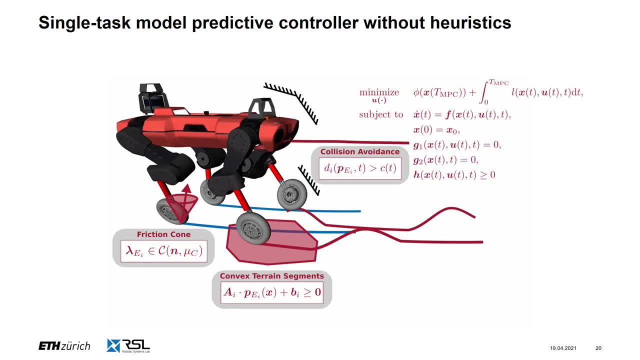 So I think we can close. I thank you very much for your talk. I think you left your contact information in case somebody wants to reach out. And good luck for your future endeavors And thank you very much for the talk. Yeah, Thank you for inviting me. See you, Bye-bye, See you. See you all next week.